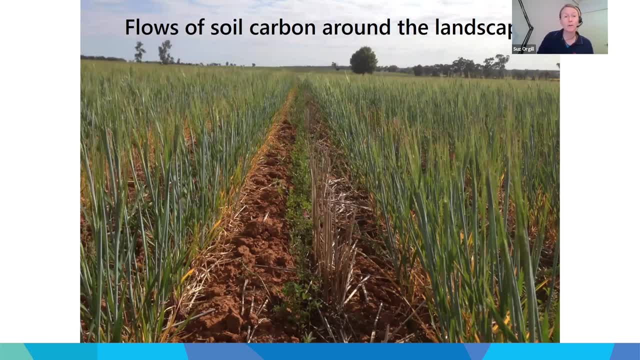 BLARm, Your own individual farming systems situations, you can think about what some of the likely practices are to impact soil organic matter cycling and soil carbon accumulation. So we're going to start with talking about the flows of carbon around the landscape. So- and someone mentioned Christine Jones earlier- I think, Anne, you mentioned that. 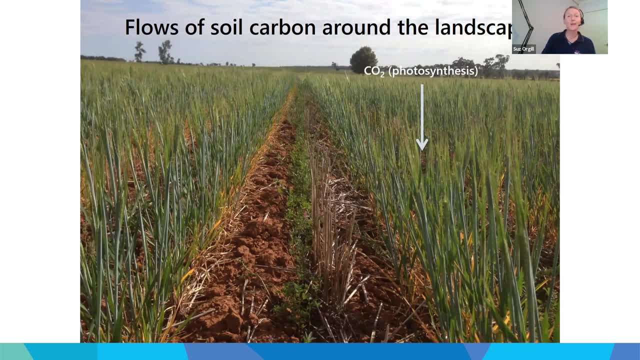 and Christine has a beautiful way of describing, I guess, the liquid carbon pathway. So where we have carbon dioxide in the atmosphere and, through the process of photosynthesis, plants take that carbon dioxide and it goes from a gas and they combine it with sunlight. using sunlight, they 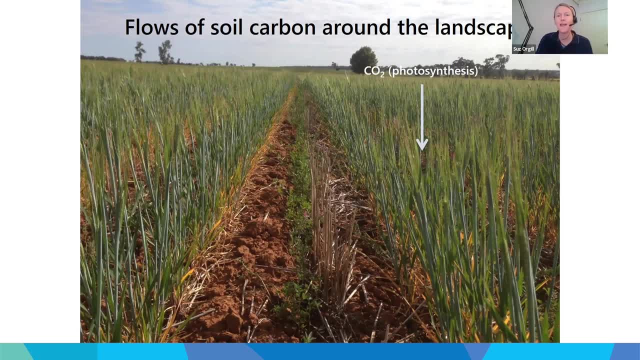 combine it with water and make energy for themselves, And this is the direct way that carbon goes from being a gas in our atmosphere to being liquid carbon in the plant and solid carbon in those plant structure as well. Once we have that carbon in the plant, it can be the 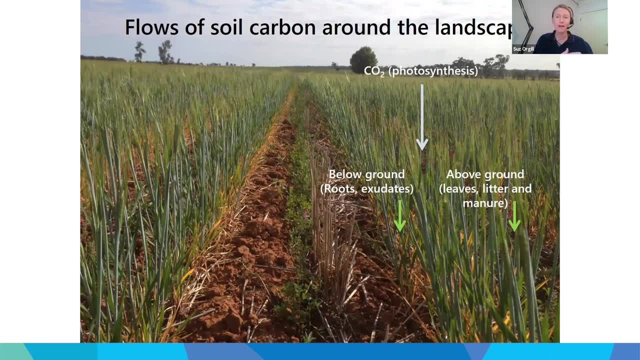 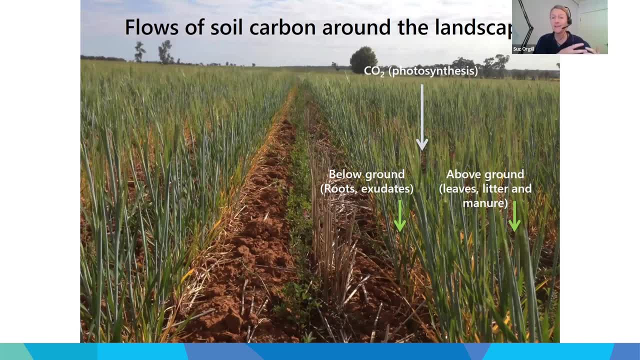 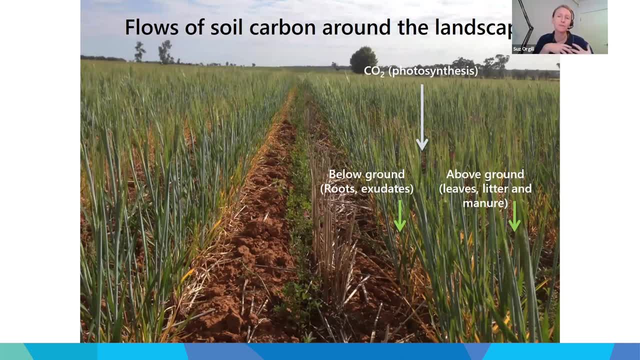 ground. about half of it leaks out of the plant root systems in the form of root exudates. So those carbohydrate rich materials which draw soil organisms into the rhizosphere to help the plant grow and explore the soil, to cycle nutrients, to mediate temperature and moisture and pH. 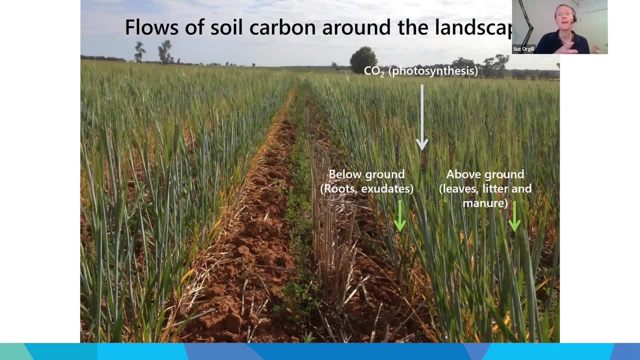 and that's a really important use of carbon in this, I guess, economy where the plant trades carbohydrates through its roots for microorganisms to help with that organic matter cycling, And we'll talk a little bit more about that as we progress. today We've also obviously got carbon stored up in the root. 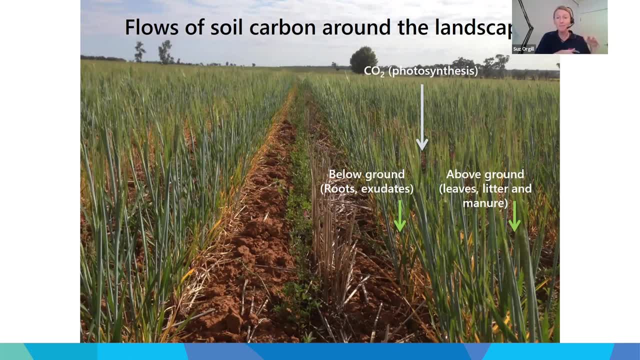 systems and different plants have different rooting depths and different root morphologies, So they're structured differently so they can put carbon at different places within that soil profile. Once we're in this medium, so once organic matter, be it from leaves and litter on the soil surface and manure to roots and exudates- we're talking about the soil organic matter pool. 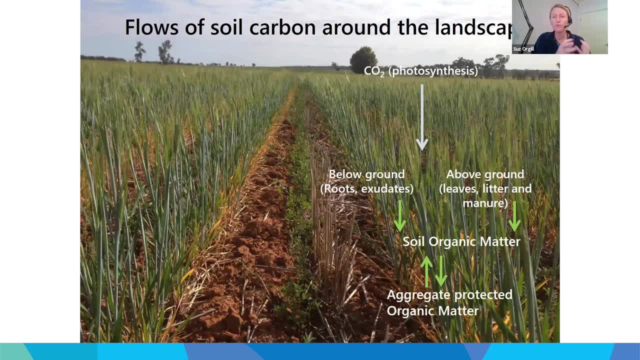 Organic matter in the soil can be protected when it's wrapped up nice and tightly within soil aggregates- so crumbs of soil. And when we say it's protected, it's protected to a certain extent from further decomposition. So we might take a soil sample, bring it back to the lab and we dry it and we grind it, we sieve it through a two mil sieve and then we can measure it and we can look at the type of carbon it is. 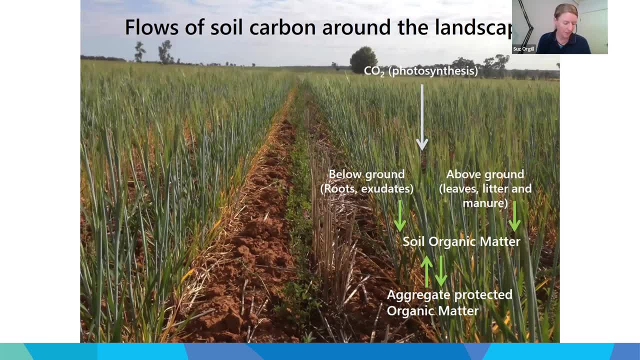 And we might say that it's labile carbon, And I think someone- maybe Cole- mentioned labile carbon in his introduction. So labile carbon is the fresh, readily decomposable carbon And that's what we might measure back in the lab. 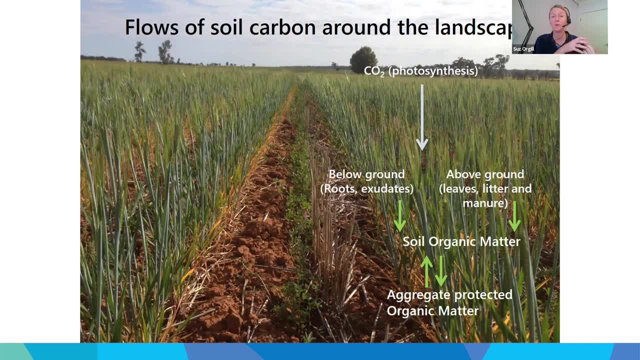 But realistically, when we're thinking about it in the soil it was wrapped up, Wrapped up nice and tightly within a soil aggregate. It was in the soil profile, so it was already protected, And say that was under perennial pasture or under a no-till system. 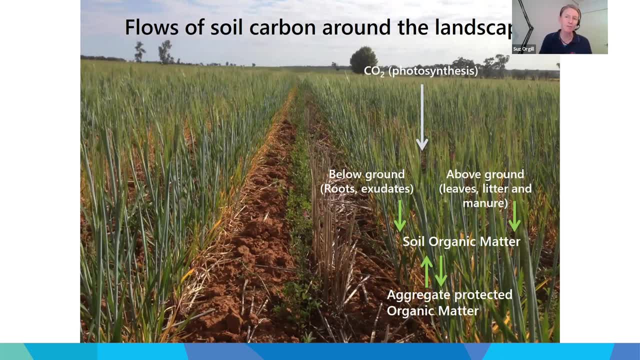 While we might measure it as labile and maybe give it a tag of being turned over within weeks to months in the field, our studies have shown that this organic matter, which is labile, could actually stay there for a matter of decades, which is really important to think about. 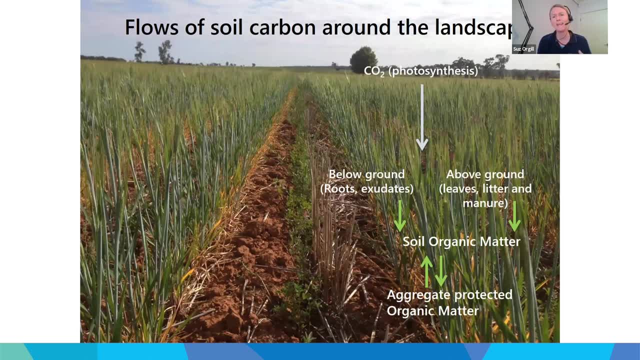 So, straight away, there's a role for our land management in protecting carbon that's stored. But we also like our carbon to be our organic matter, to be functional, because it feeds our microorganisms And I said, as I said before, that's a really important pathway for nutrient provision for our crop and pasture growth. 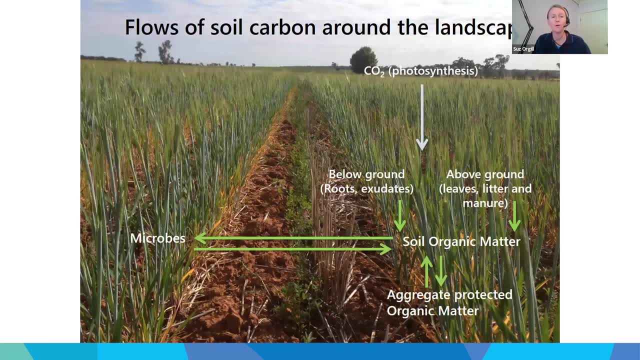 And it also promotes and enhances soil structure as well. So our microbes, as well as our other soil critters, will decompose organic matter, And nearly all of our plant-available nutrients need to grow through this cycle to become available, So it's certainly something that we need to, I guess, appreciate. 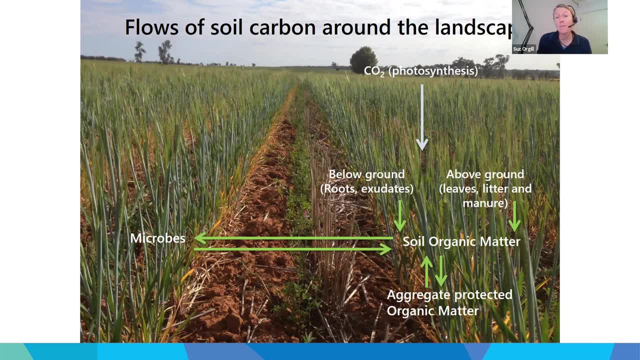 And it's a really important use of organic matter. Now, microbes themselves are a type of carbon in soil, So we can measure that through our microbial biomass carbon And it contributes to the total carbon pool when we look at that in our soil test as well. 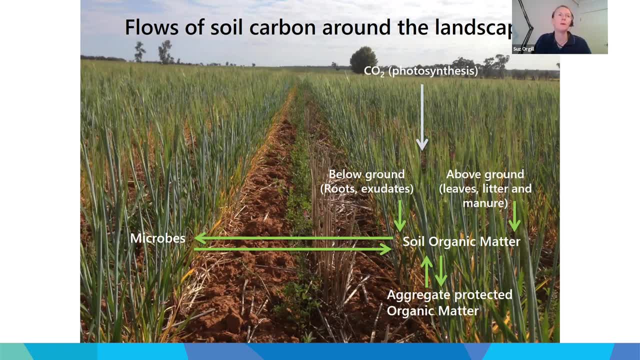 Humus, which is a form of carbon that you'd be familiar with, is basically dead microbes and microbial products, And so the more, The more microbial action we have, the greater the extent we can build up humus in our soil as well. 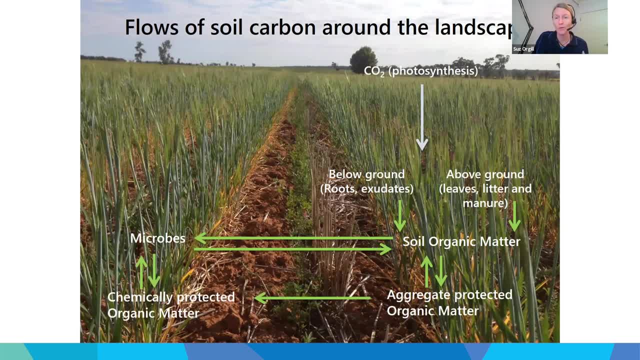 Now, microbial products can also be stabilised in the soil through either their form, so their nutrient relationships and the nutrient ratios of their form, but also through their association with clay particles as well. So some of our humic and fulvic acids can form really neat bonds with clays. 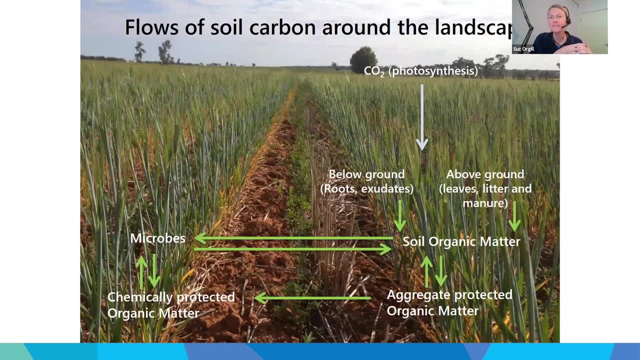 And this is called organomineral association. And again, this is another way of stabilising carbon in our soil, which leads to building up carbon within our soils as well. So if we were just to have a look at this system, we could think: OK. 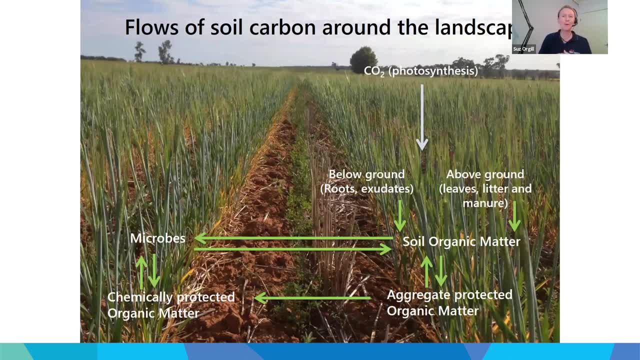 if we've got rainfall and if we can grow as much biomass as we possibly can because we've got good tactical agronomy. we're looking at promoting soil cover. we're enhancing soil structure. we've got diverse either rotations or substrates. we're enhancing soil structure. we've got diverse either rotations or substrates. 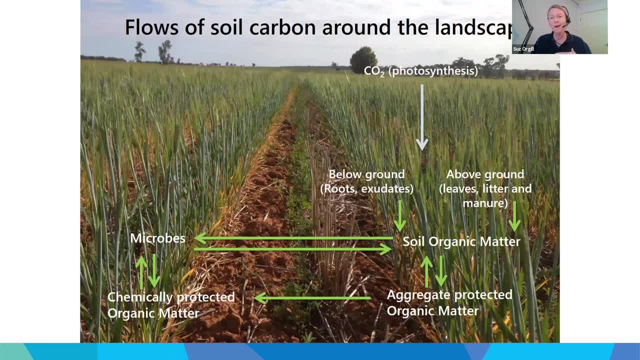 species being planted in our pastures, we're maximising that photosynthetic pathway which increases the amount of carbon which can go into the soil and can increase the residence time or the build-up of carbon. Now, when this carbon builds up in the soil, as I said, it can be in different fractions. 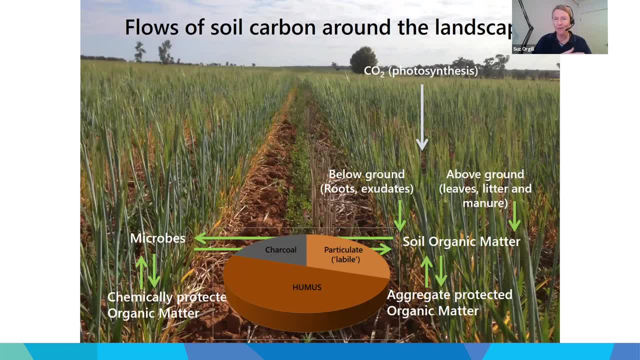 So we have our particulate or our labile carbon, which is kind of like the cash flow. So that's the readily decomposable fraction which is really important for energy and for the soil And that's where we have our microorganisms. 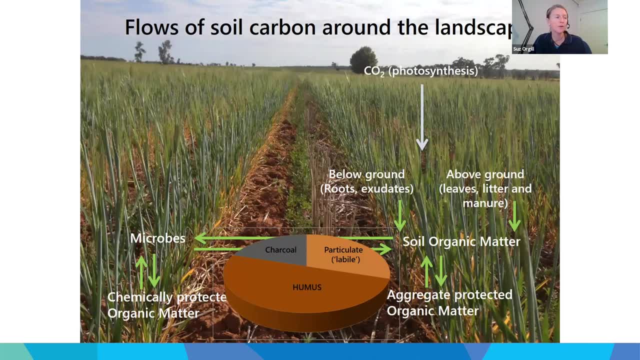 We have our humic pool which, as I said before, is those microbial products which build up in the soil and different cells and parts of microbes which build up into a very important nutrient reservoir because they're very nutrient rich and a very stable form of carbon. 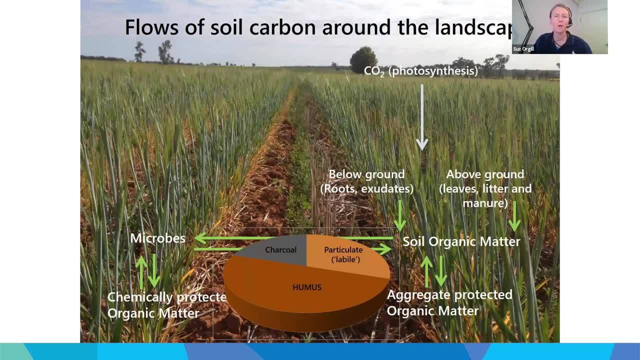 And then we also have another stable form of carbon in our soil in terms of- I've called it charcoal here. It's technically called char, but it's very, very fine bits of charcoal that you wouldn't see in the soil, It wouldn't be visible to the naked eye- which occur in our soils to varying extents, but up to 35% in some places, have been reported. 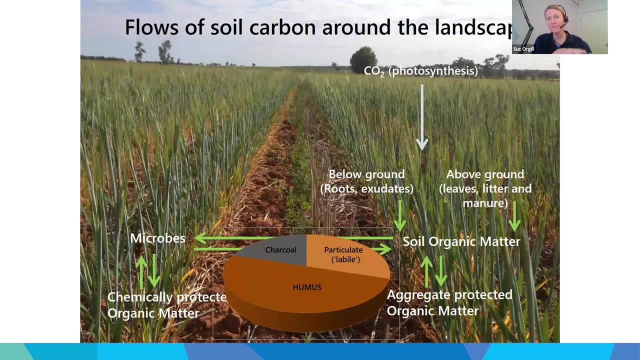 And this is through patterns of tens of thousands of years of burning across the Australian landscape, So not necessarily accumulating through burning stubble, but we're talking about big burning events which have happened over tens of thousands of years. We also have a carbon loss pathway in this flow as well. 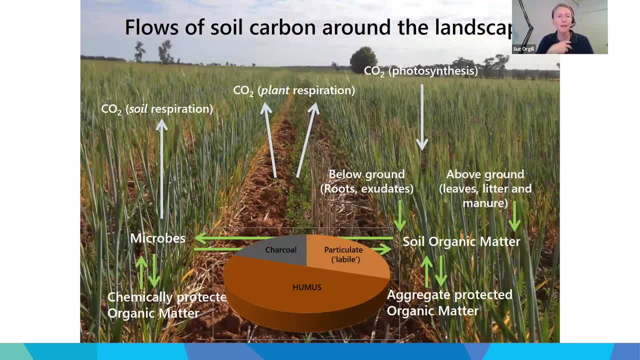 So as our microbes decompose organic matter, they respire just as we kind of. when we're active, we respire as well. Actually, even if you're inactive, you'll respire, hopefully, And plants will respire as well. 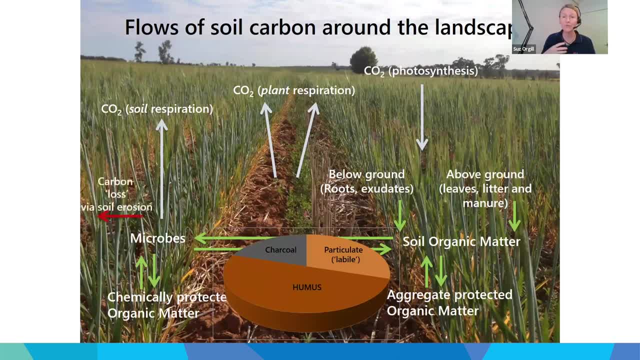 The other pathway that we have for loss is through erosion, And what this means is that we can have soil, organic matter, be physically removed from the site, And now it might move to a place in the landscape which makes it more vulnerable to decomposition, or it just might move somewhere and be buried. 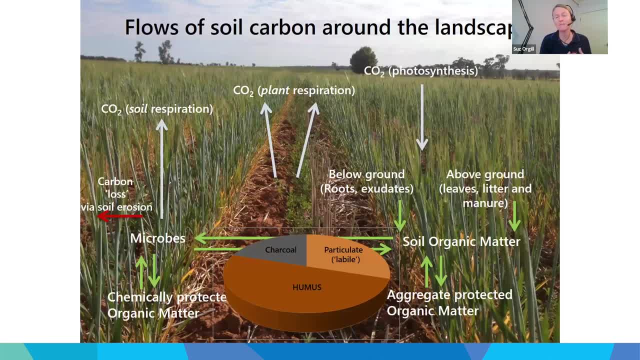 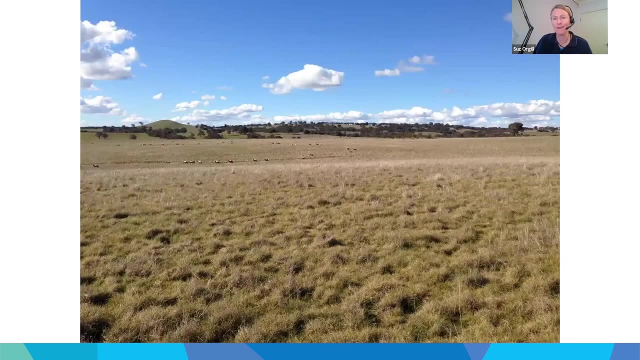 So it doesn't necessarily mean that it's going to go back up into the atmosphere, but it's certainly a loss from that site And that's certainly something, through promotion of ground cover and minimum tillage, that we can mediate or reduce Now that flow of carbon is happening in all of our landscapes. 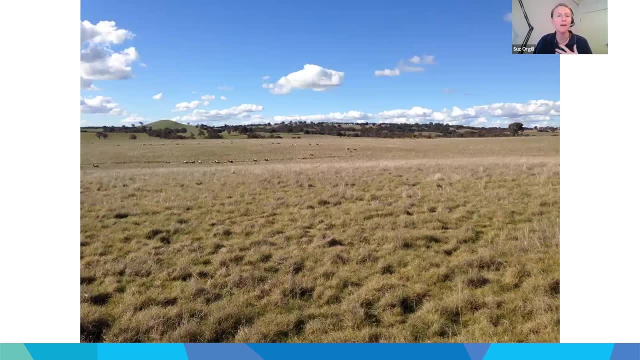 So the picture in the previous slide was a cropping landscape. This is an introduced permanent pasture around Booroa. That flow of carbon is occurring in this landscape as well. What we can influence is the magnitude and rate of that flow with our land management. 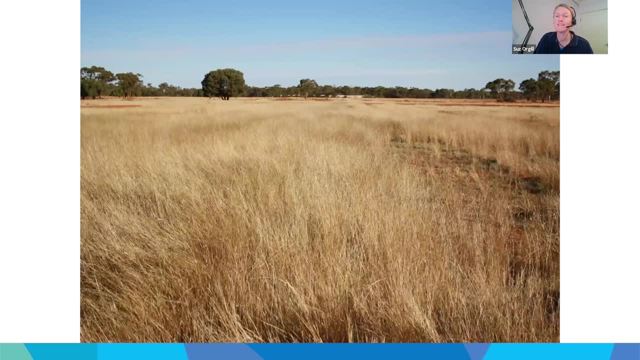 Similarly, in this environment here, which is in the rangelands, and this is a mitchelgrass pasture out near Cobar- the same flow is happening. I guess the levers that we can influence, though, are the things that will change. 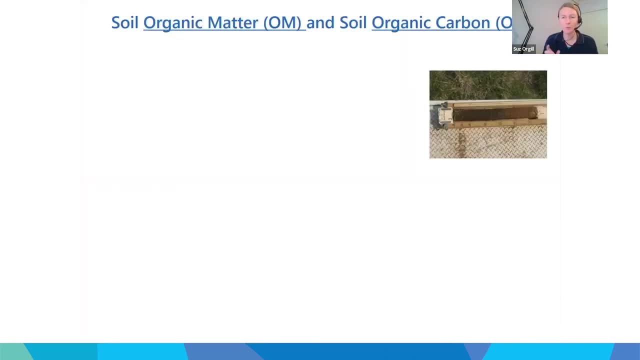 Now I've used a couple of terms interchangeably And I just want to touch on a few definitions. So we have soil organic matter and soil organic carbon. When we're talking about soil organic matter, by definition we're referring to the fraction that's less than two millimetres in diameter. 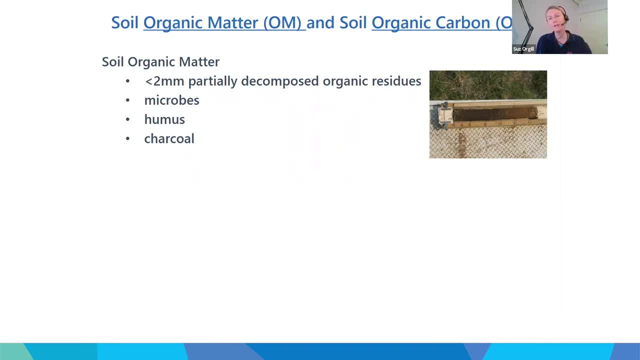 So you might recall in the previous slide where I said: we take a soil sample, we dry it to 40 degrees and then we sieve it through a two mil fraction sieve. Now, when we're including the greater than two mil fraction, it gives really high. 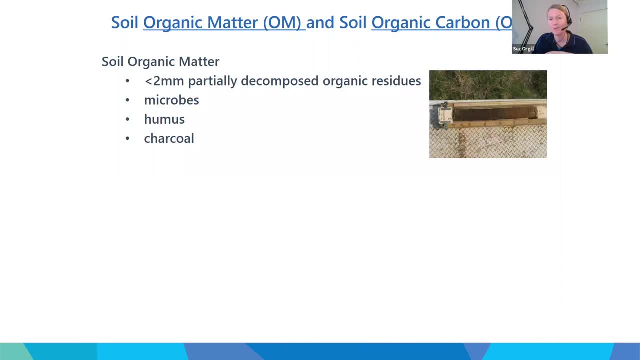 highly variable results. when we're looking at total carbon results Also, the less than two mil fraction is the fraction that's more closely related to our soil property. So it gives us a good indication, I guess, of the soil organic matter that can actively influence those soil factors. 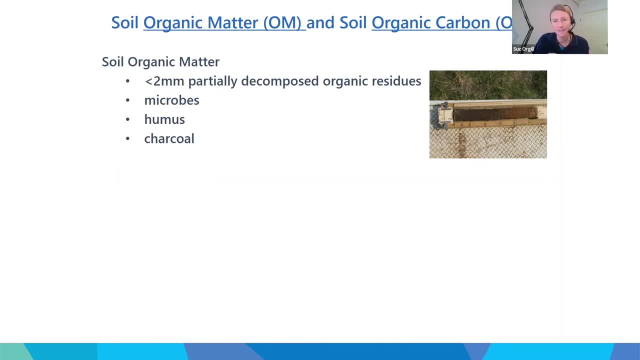 So that's why we look at less than two millimetres. It's also really important for standardising across labs, So it has a role there as well. Now, once we're looking at the less than two mil fraction, it includes mostly decomposed organic residues, microbes, humus, charcoal. 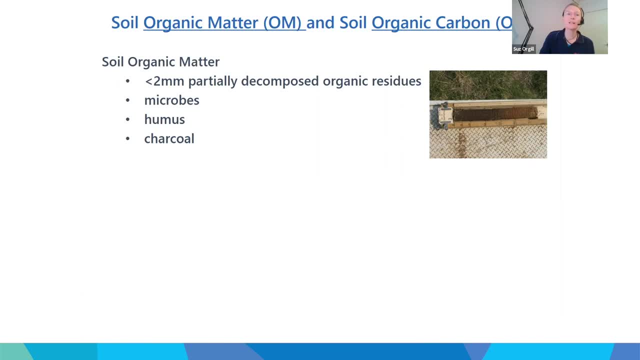 So it includes all of that. Now, when we look at soil organic carbon, carbon is the measurable component of the soil organic matter pool, So soil organic matter is approximately 58% carbon by weight. Really importantly, the rest of organic matter is made up of all of these plant nutrients which we're used to talking about in our recipe agronomy. 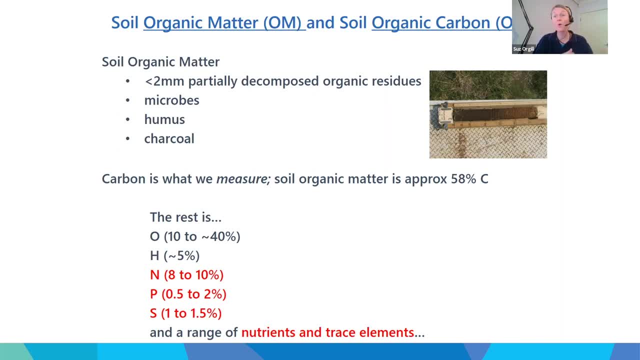 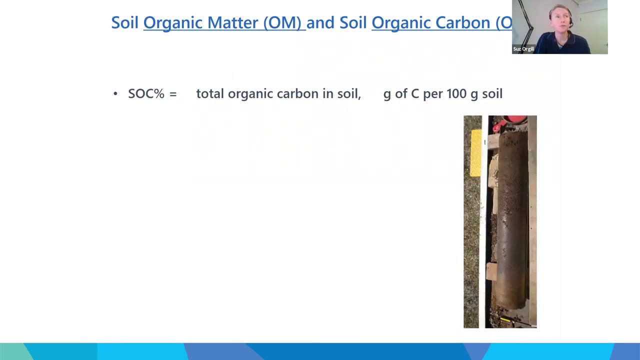 So nitrogen and phosphorus and sulphur, So soil organic matter. while it's carbon, it's also a really important nutrient reservoir as well, And there's a range of trace elements which are in that pool also. Now, when you get your soil test results back from the lab we like to look at, well, first of all, we like it to be a NARTA accredited lab. 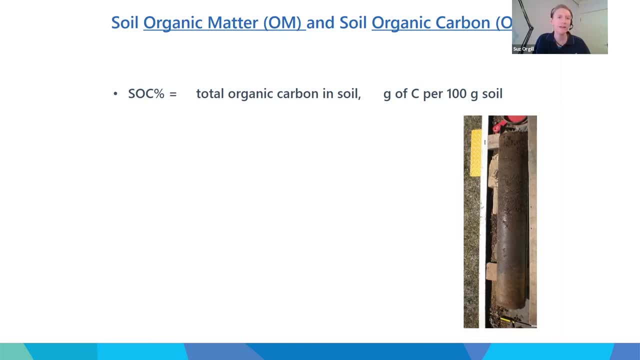 So we like it to be, so that they're using standardised procedures. It needs to be on the less than two mil fraction which NARTA accredited labs will use. And then we look at the soil organic carbon percentage. Now some labs will also report soil organic matter content and that's a calculation. 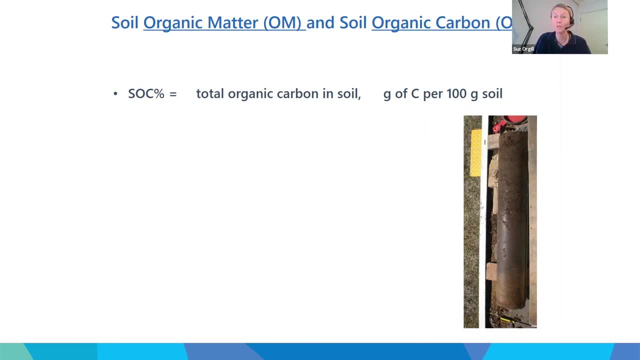 So that's where they'll take your organic carbon percentage and multiply it by a factor 1.72, to give you organic matter. So let's cut the calculation out for this one and we just look at soil organic carbon percentage And this is the total organic carbon that's in the soil. 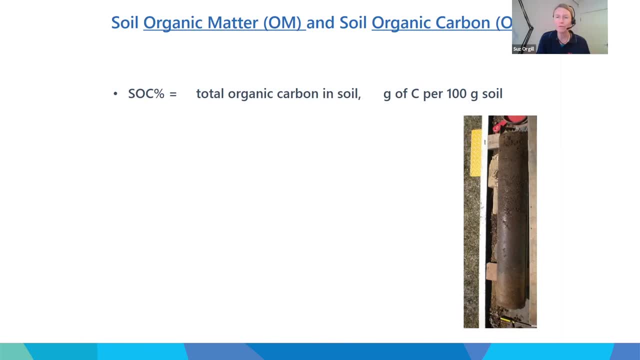 So that includes all those pools that I spoke about. It includes all of those: the char, the humus and the labile carbon. It might be reported in grams of carbon per 100 grams of soil and that's the same unit that directly can be converted to percentage. 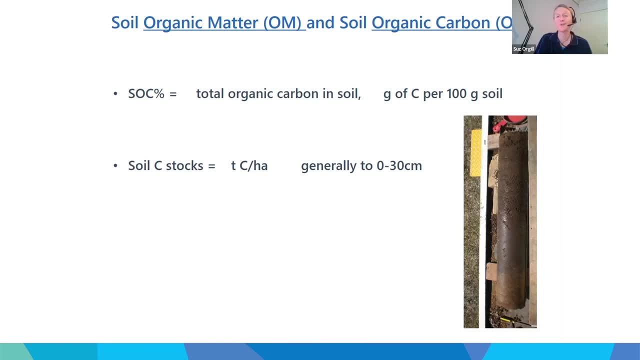 Now, something else that we'll talk about throughout this presentation is soil carbon stocks, And this is where we're looking at the tonnes of carbon per hectare, And typically this is reported to 30 centimetres, because that's the international protocol. 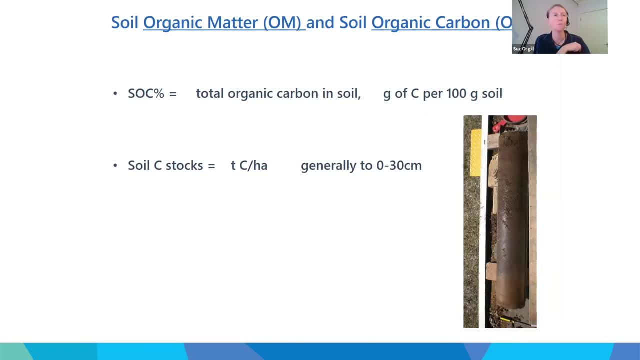 For carbon trading, And that's, I guess, become the adopted standardised way of reporting soil carbon across different soil types and land uses. Now, this is a calculation, So it uses that soil organic carbon concentration that I've just mentioned. It uses the bulk density of the soil and the depth of the soil to give you that tonnes of carbon per hectare. 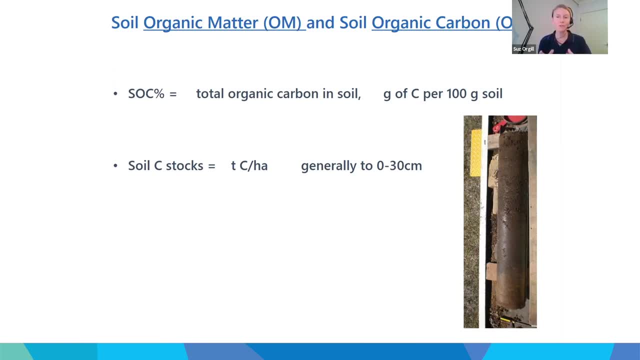 So we take a concentration, We know what the mass of the soil was and the depth over which that occurred, And then we can compare that to what we've already observed. So, as a result, we're able to move from normal soil to carbon dioxide relative to the mass or the quantity of the soil in different days. 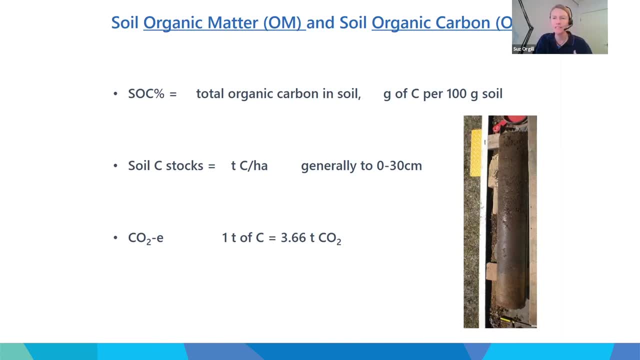 Another unit that often gets spoken about with with soil carbon trading is carbon dioxide equivalence. Now, one tonne of soil carbon is equivalent to 3.66 tonnes of carbon dioxide, So this is just a metric unit that it's really important to think about how you're reporting your carbon results, and it needs to. 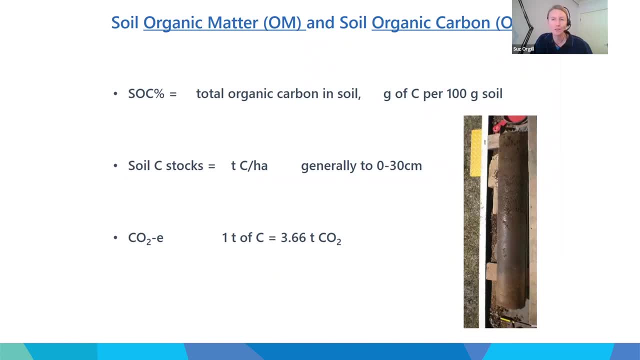 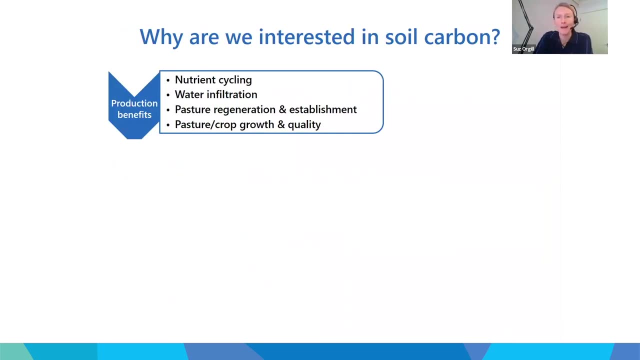 be fit for purpose. So generally it's going to be in concentration or soil organic carbon stocks. So why are we interested in soil organic carbon? And it seems like a silly question to ask a group like this because you've already answered it. It's really important for nutrient cycling. It's 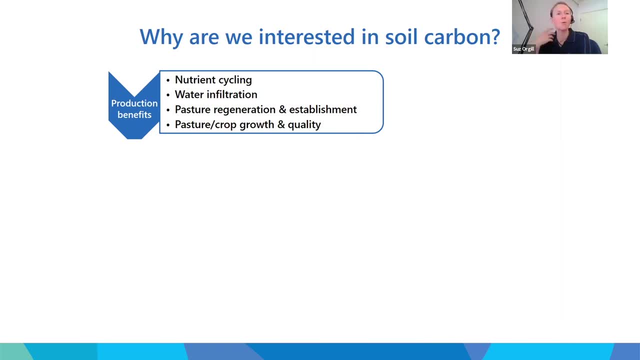 important for pasture regeneration, It's important for crop and pasture growth and quality. So there's these immense production benefits And some of these immense production benefits are directly related to the soil factors that soil organic matter can influence. So increasing your soil organic carbon can also can increase your cation exchange capacity. So the cation exchange 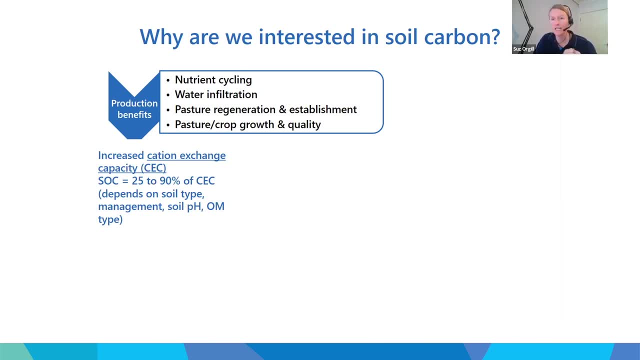 capacity is the soil's ability to hold on to an exchange nutrients And, in particular, what I like to refer to as your EM. so calcium, potassium, sodium, magnesium, aluminium, and they're our main cations that we're talking about. 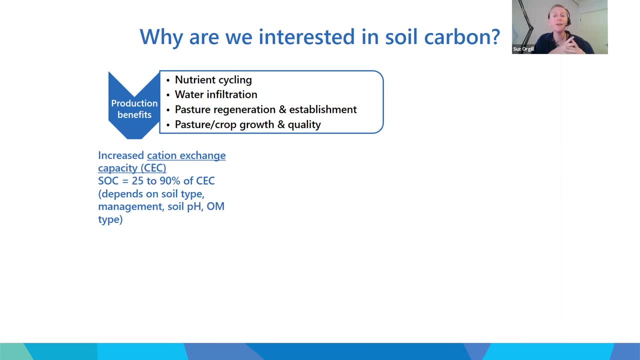 Now in a clay rich soil, so sorry. cation exchange capacity is mainly influenced by two things: the amount and type of clay and your soil organic carbon content. Now, in a sandy soil, your soil organic carbon content is the amount and type of clay and your soil organic carbon content. 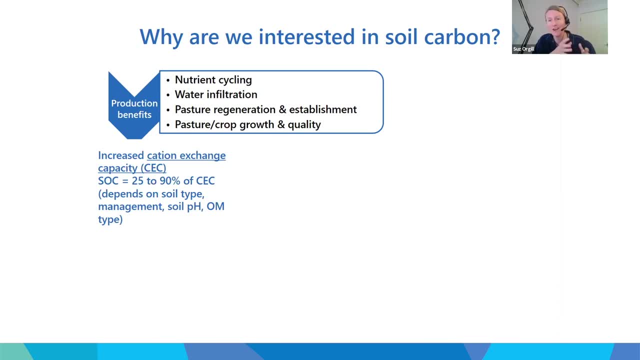 So your soil organic carbon can account for up to 90% of that cation exchange capacity. So it's really important, So it's a real driver of, I guess, nutrient storage And cation exchange capacity is going to be dependent on soil type and management, soil pH and also the organic matter. 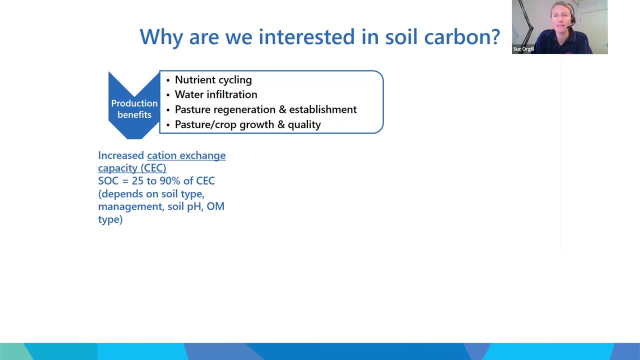 type. But when we're thinking about cation exchange capacity- and I used this example yesterday as well- I want you to imagine that we're all sitting in a big room full of people and we're all sitting in a room full of people. So we're in a room and that room is our soil- All the chairs that are laid. 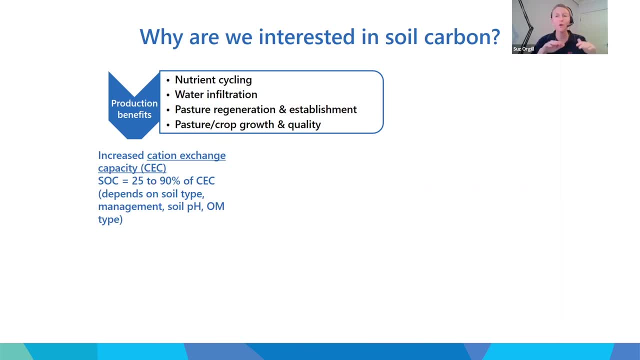 out is our spaces on our clays to hold on to our EMs, our cations, And all the people sitting on those chairs are our cations. So calcium, magnesium, potassium, aluminium and sodium, And that's what we've got. That's our soil. Now, what we're talking about is, with increasing soil, 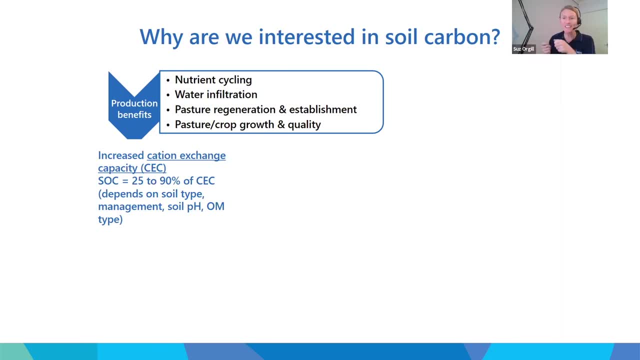 organic carbon is bringing a whole heap more chairs into that room. So we're talking about that room. So now, all of a sudden, we can have more people sitting down right, So we can have a greater nutrient storage in our soil. Now, if we look at the flip side of that, if we take away 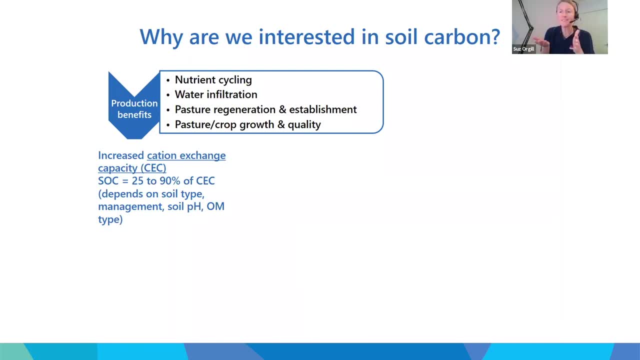 half the chairs that are in the room. now half the people are standing. they're not attached to the soil anymore, they're standing. What happens when it rains? They get leached away. So they're now in soil solution. So they're not actually held within the soil, they're in solution. So the importance. 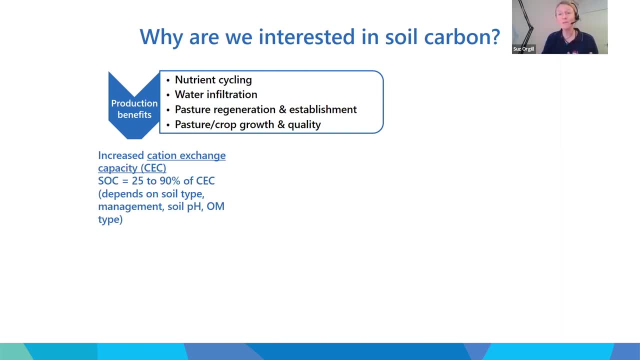 of organic carbon is that we're going to have a greater nutrient storage in our soil, So we're carbon- is that we can increase the soil's ability to hold on to and exchange nutrients, which is a really important function. It's still important in clay rich soils, but it's incredibly important. 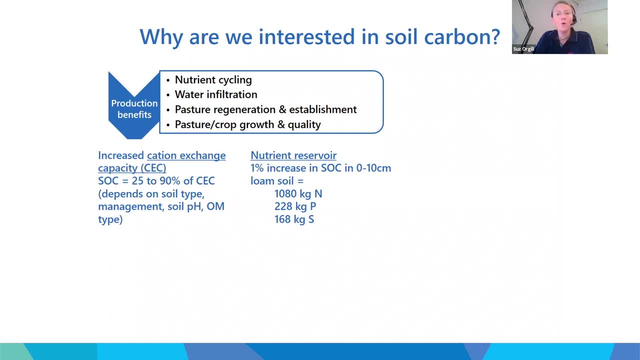 in sandier soils. Now, soil organic matter is also a really important nutrient reservoir and I mentioned that a couple of slides ago. but in general, a one percent increase in soil organic carbon- so going from a carbon percentage of one to two in the top 10 centimetres- gives you over a. 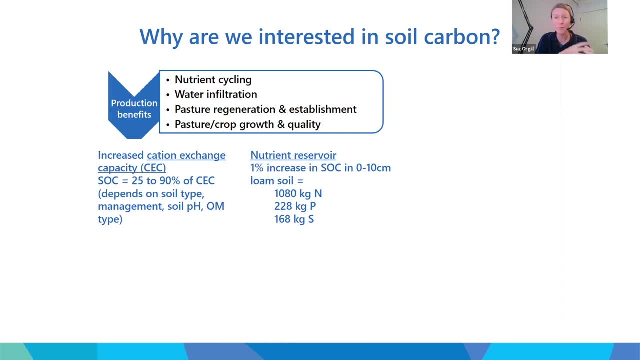 tonne of extra nitrogen, So that's really important straight away. we're talking dollars here, so a tonne of nitrogen, 200 and something kilos of phosphorus, 160 something kilos of sulphur. so it's really important in terms of the productivity and benefits of those nutrients as well. So with that soil, 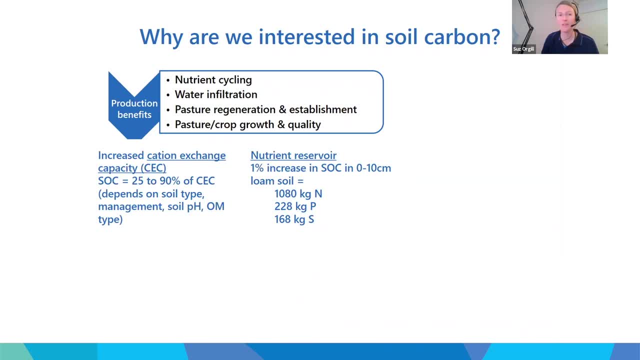 organic matter comes nutrients and there can be a value associated with that. And remember what I said before: nearly all of our nutrients need to first pass through soil organisms to become plant available, and this is where organic matter supplies not only nutrients but the energy for microorganisms to provide that function. 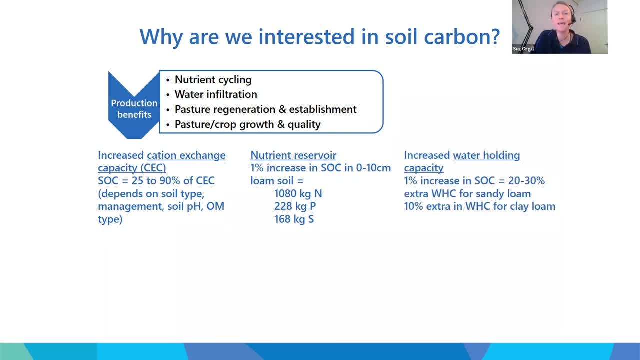 Another really important function of soil organisms is through increasing water holding capacity and infiltration, as they decompose organic matter. So as soil organisms decompose, they decompose organic matter. So as soil organisms decompose, they decompose organic matter. They produce sticky substances which stick particles together and enhance the structural 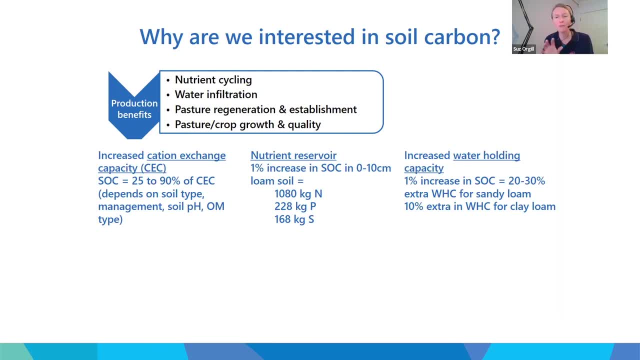 stability of the soil. Fungal hyphae will wrap up soil aggregates, making it so that when it rains that soil doesn't collapse. it holds together and acts like a sponge for increased water holding capacity. In sandy soils this is really in clay soils it's important as well, but particularly in 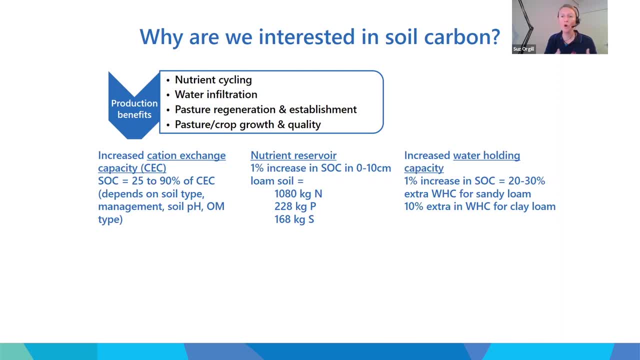 sandy soils, it can have a great effect on the total water holding capacity of those soils. So a 1% increase, if we use the previous example, going from a 1 to 2% soil organic carbon reading, can give you up to a third extra capacity to store soil moisture. When we're looking at our 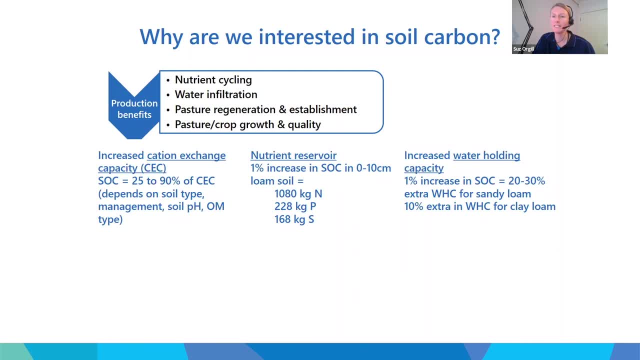 fluctuations in climate and the variability that everyone's experiencing, making use of all the rainfall that falls on properties is really important. So when we get a 50 millimetre downpour out at Wagga, making sure that that 50 millimetres goes down is really important. 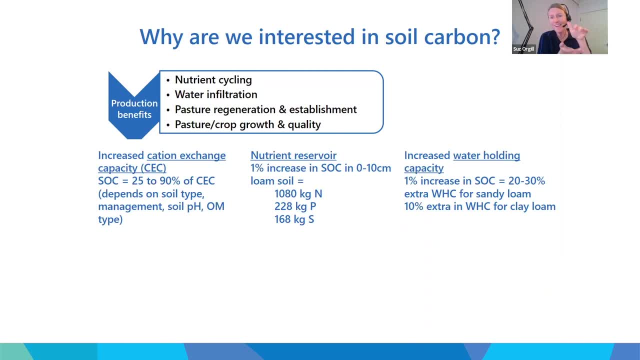 When we get a 50 millimetre downpour out at Wagga. making sure that that 50 millimetre goes into the soil and is stored there again is so important for productivity, And this is what we call our functional carbon. So it's not just about getting organic matter into the soil and keeping it there. 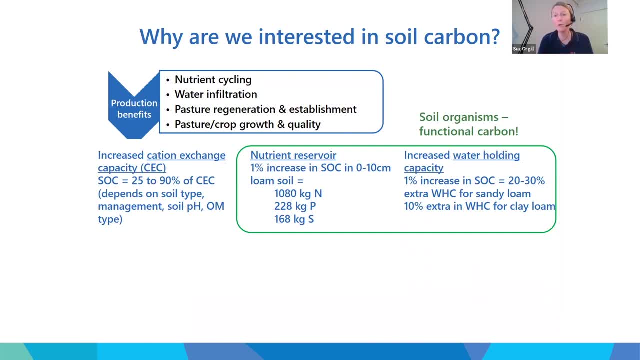 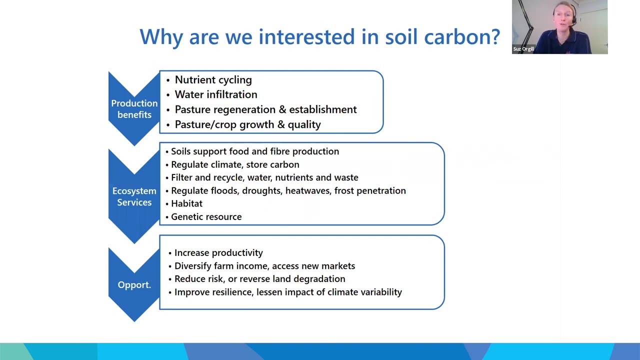 it's also about that carbon economy, because that microbial process of reducing or mineralising and immobilising nutrients and enhancing water holding capacity is really important. Now, through these things, we do have to look at different types of services. So there's the provision of off farm. 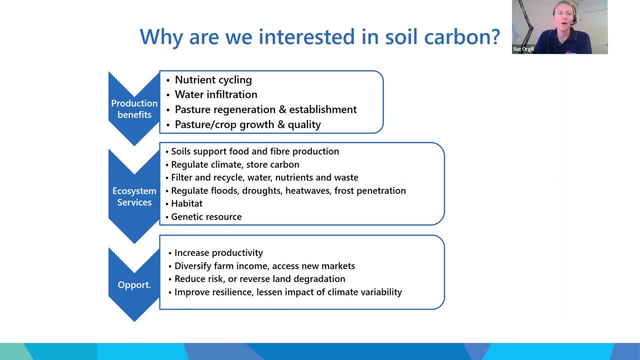 services, so ecosystem services. So there's things like regulating climate, There's things like filtering and recycling water and air and nutrients, And these all have a value for our society as well. There's increasing opportunities, I guess, to diversify farm income through documenting the benefits of. 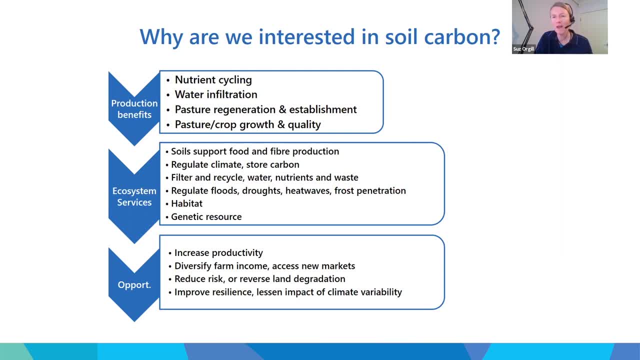 improved land management for some of these ecosystems. So we're looking at really looking at those technologies that we use. So we're looking at the solutions that we're looking at through the ecosystem services. So what we're talking about there is collecting the information that 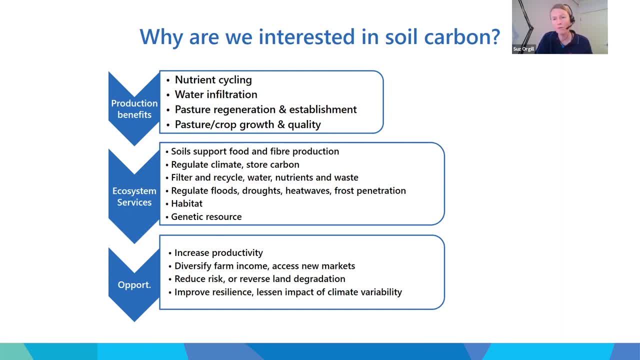 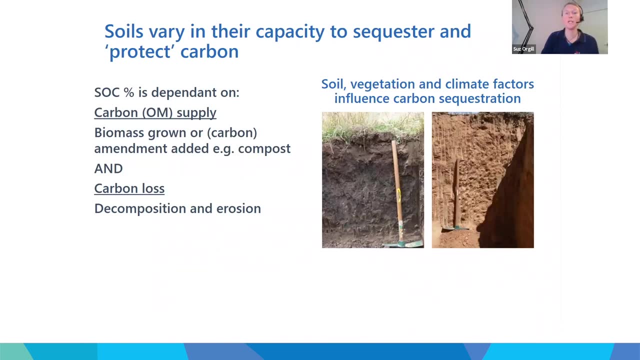 demonstrates the public good benefit of on-farm management. And we now have emerging markets, not just the carbon trading ones, but emerging markets where that's going to be valued, So that can be a farm product as well. So when we think about our sequestration potential, we know that. 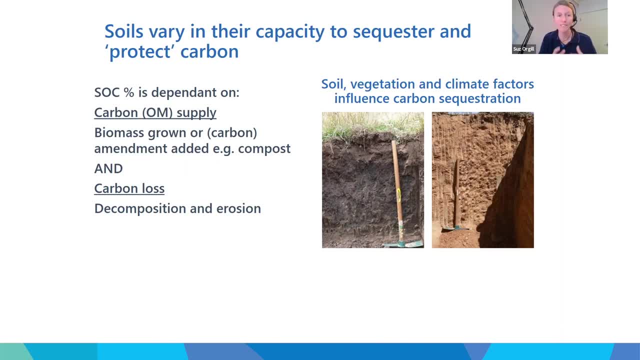 our soils vary in their capacity to sequester and protect carbon. If we're looking at just the balance, though, our soil organic carbon concentration is dependent on the amount of organic matter going in. So it's either grown in situ or it's grown somewhere else and brought to. 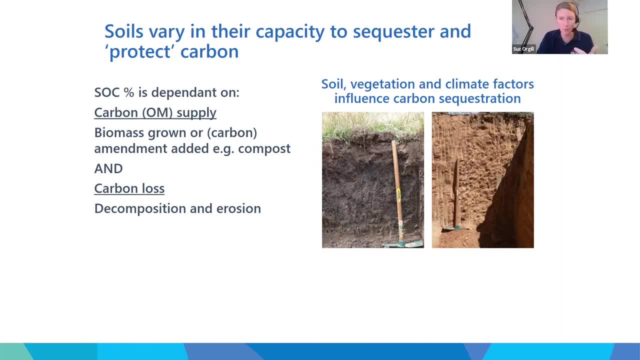 the site in terms of hay, compost, biosolids, manures, And that's balanced by the carbon loss, And the carbon loss is the respiration from decomposition, So the loss of carbon that way, or from soil erosion, where we've got that physical removal of carbon from the site. 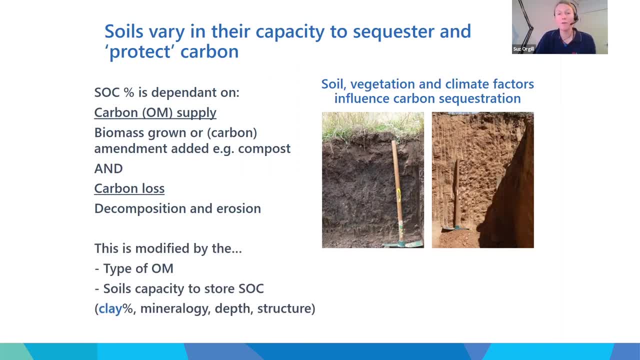 there Now that balance is going to be modified by the type of organic matter that goes into the soil. So not only its physical structure, which influences the surface area for microbes and other soil organisms to decompose it, but also the nutrient composition of that, the carbon to 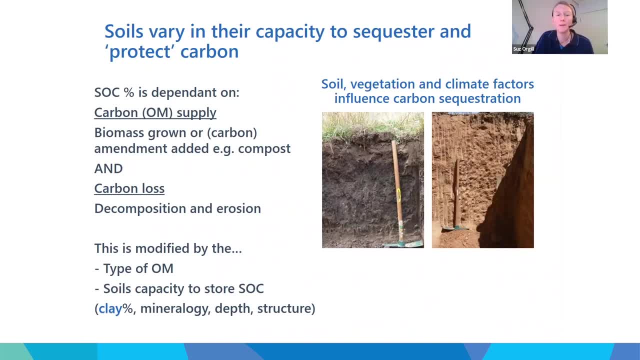 nitrogen ratio. But also the soils can be decomposed by the type of organic matter that goes into the soil. So that's what we're looking at here. So that's what we're looking at here. So this is dependent on things like the amount of clay, the type of clay, soil depth and soil structure, And 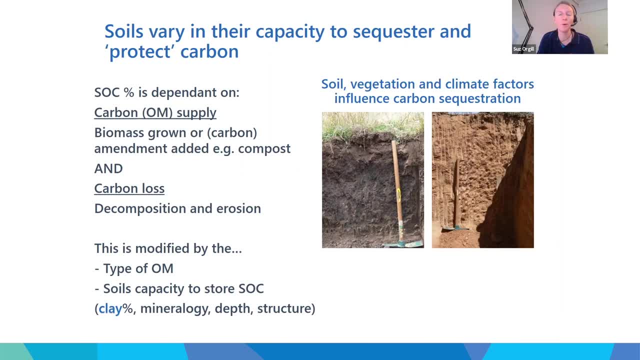 they can all modify that flow of carbon that we spoke about on the first slide. Now, some of these factors, or all of these factors, drive productivity. Some of these factors can be changed. So with our land management we can change the type of plants that we're growing. 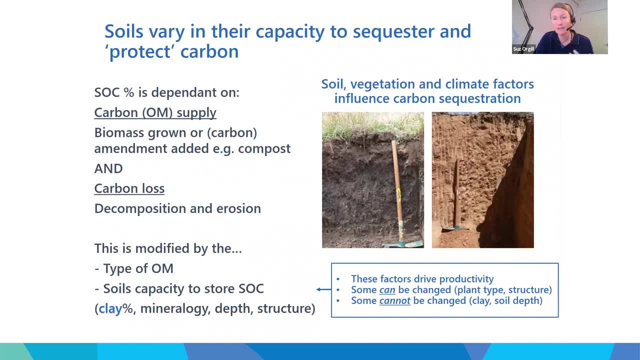 We can implement practices that we're doing. We can implement practices that we're doing. We can implement practices that we're doing. We can implement practices which enhance and protect soil structure, And some can't easily be changed, So, in particular, the clay content and soil depth. 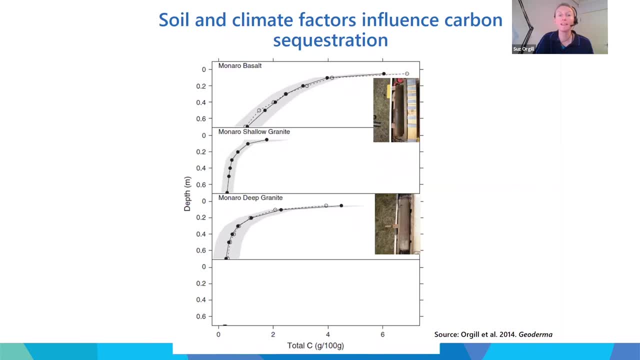 If we look at just how much these soil and climate factors can influence carbon sequestration. I just wanted to share this graph with you. So what we're looking at here is: on the X axis, we've got our total organic carbon percentage. It's in grams per 100 grams. Remember, that's just percentage. And on our 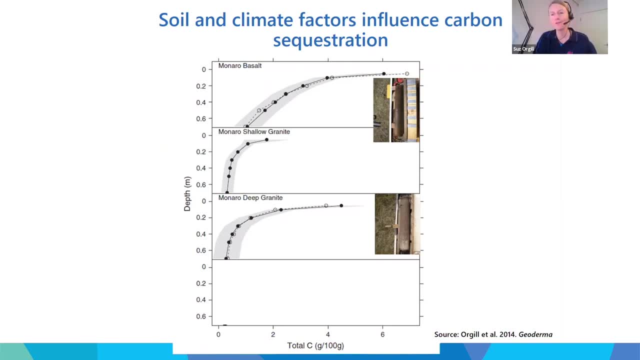 Y axis we've got depths descending. So for soil scientists we'd like to have the soil surface at the top of the graph and then it goes down with depth. So it's going from the soil surface at the top down to 70 centimetres. Now, the three graphs that you can see there are for three different. 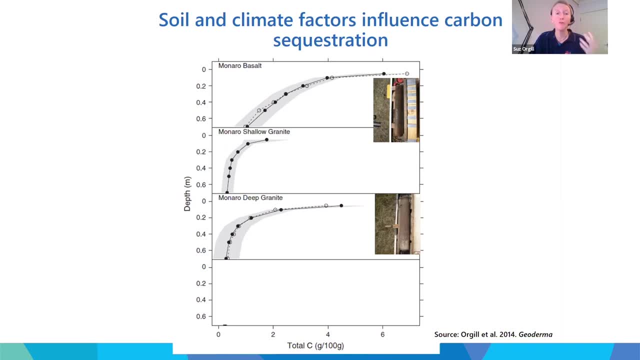 soil types in the same region. The first graph, the top one, is for a basalt-derived soil, So a very, very high concentration of high fertility clays. The second graph, down in the same region, is a shallow granite-derived soil, So this is an extremely 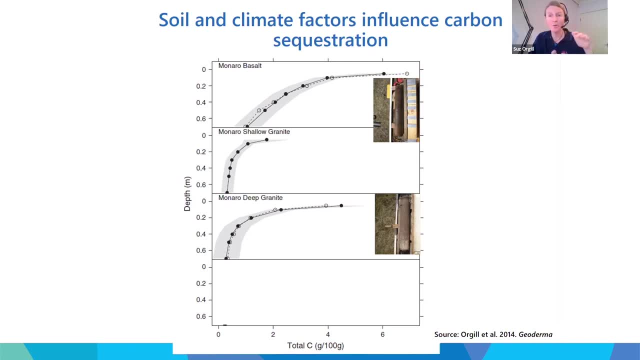 sandy soil which is poorly structured and shallow in terms of the soil depth, And the next graph down is a deep granite-derived soil, So it's heavily duplex. We've got a sand over a clay, but you've got a good depth of soil and reasonable clays in the subsoil. Now what we're looking at. 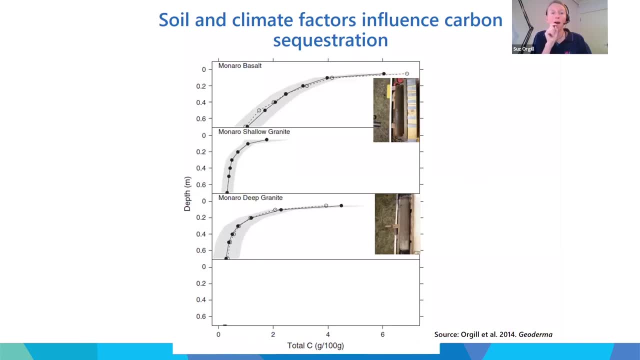 we've got two lines. There's the black line with the solid dots, and then there's open dots as well. They're different pasture types, So one dominated by native species, the next dominated by introduced species. It actually doesn't matter which is which. 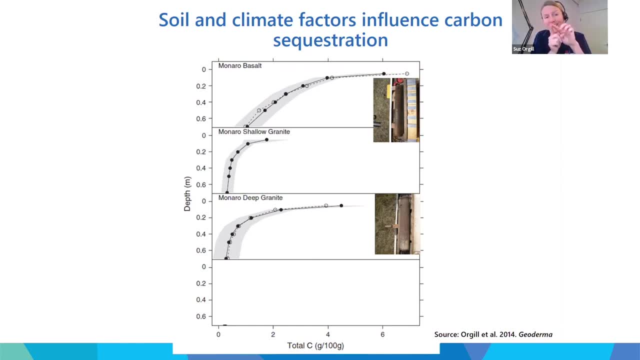 because there was no difference. Now, the grey shaded line going down, that's the range in those carbon values across 30 sites. Now, as you can see, we've got higher carbon in the top five to 10, zero to 10 centimetres, and then it declines with an. 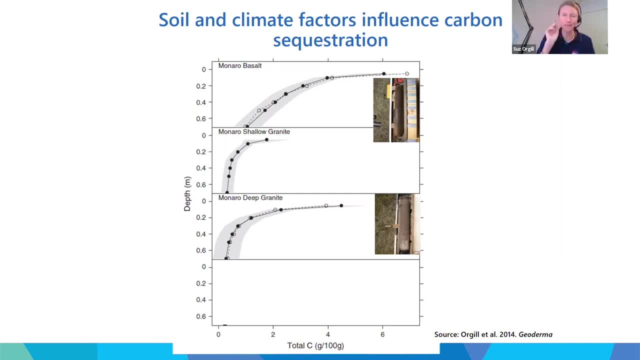 increase in depth And you see that often in a lot of our soil profiles other than when you move out west, when it's kind of less of a decline. So there's more carbon in the surface soil, less in the subsoil. Next thing you notice is that those graph shapes are very different. 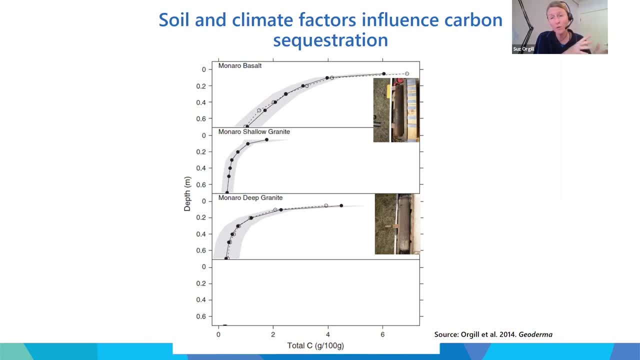 aren't they depending on soil type. So, for the same region, soil type is influencing not only the amount of carbon in the surface soil, but carbon as it goes down the profile as well. Now in these soils, when we looked at the tonnes of carbon per hectare, so the carbon stocks there. 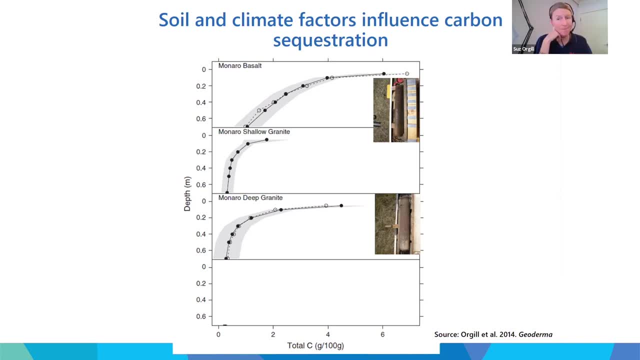 was twice as much carbon under the same pastures on basalt derived soils than there was on the deep granite derived soils. so the fertile granite soils. When we just look at the granite soils, there was twice as much carbon in the fertile granite soils compared with the 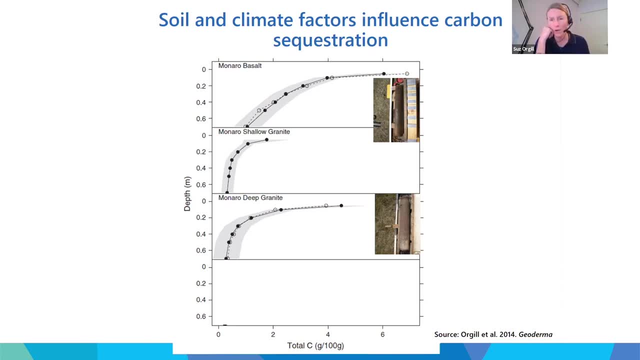 lighter textured, shallow granite soils. So soil type is a major factor in influencing carbon stocks. Now there's one graph that I had hidden there. If we look at that now. now these are deep granite derived soils. There was 24 in this survey, which is in the bottom graph here. 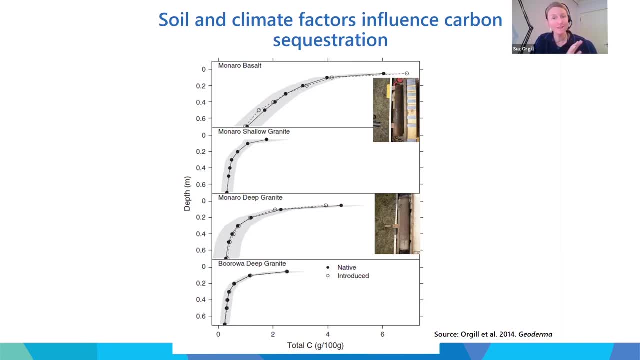 in the Booroa region. So it's a similar soil type. You can see already that the carbon profile still declines as you get an increase in depth. but also the carbon concentration was far less in the Booroa region- same soil type, different climate- than in the Monaro region. 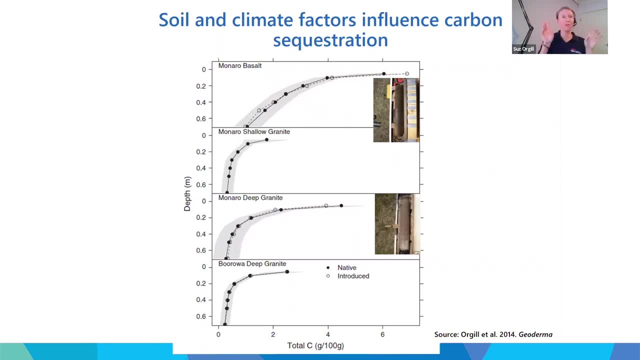 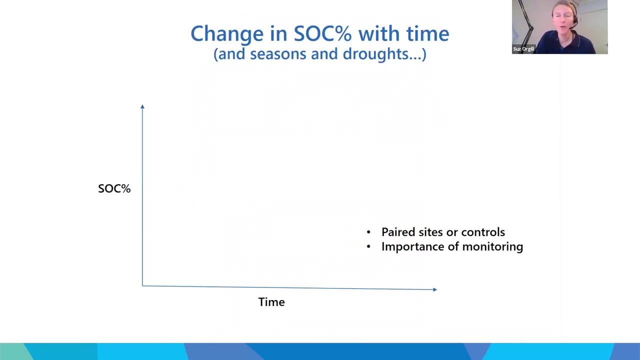 So all that was different. They're the same soil type. All of a sudden. now we're thinking about how much rainfall falls and when it falls in the season. So they're the same pasture type. So climate's also going to be really important when you're thinking about sequestration potential. Now yesterday I got asked a question. 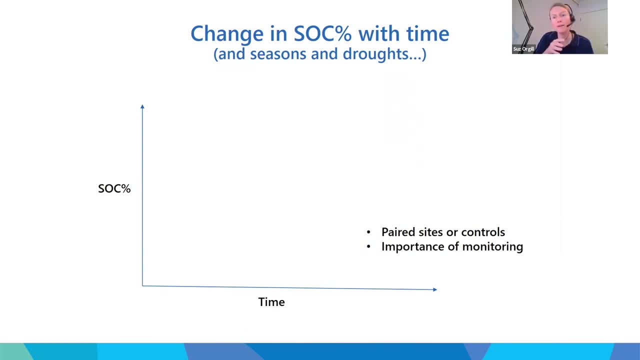 about changes in soil, carbon or the variability within a season and between seasons when we get droughts. So I just wanted to give you this. It's like just a conceptual image of what happens in the fluctuation of the soil type. It's a conceptual image of what happens in the fluctuation of the 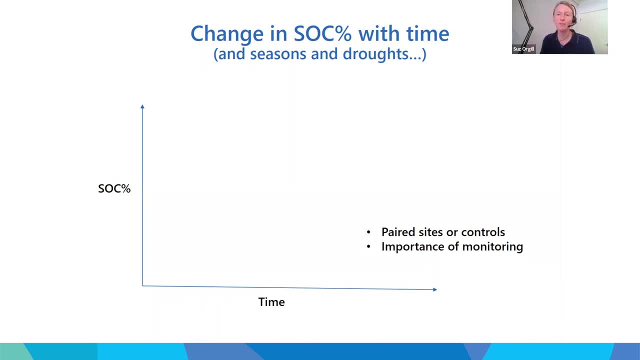 soil carbon. So here on the x-axis we have time, It doesn't matter, for what I'm going to tell you about. This could be within a season, It could be across various seasons or across decades. And on the y-axis we've got carbon percentage, so the carbon concentration. 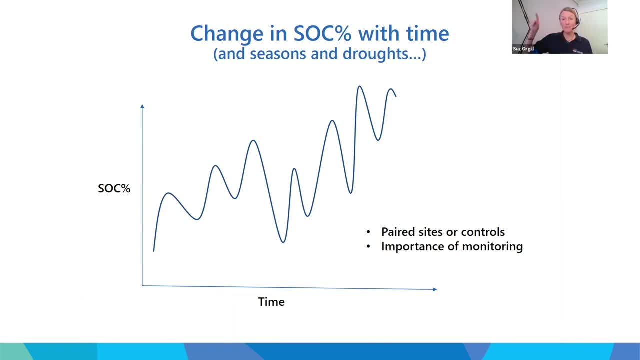 So what we'll find with time is that you'll get this bouncing around. So, because we know that carbon's influenced by biomass production, biomass production's influenced by rainfall temperature, and we know that carbon's also influenced by microbial processes, which are also 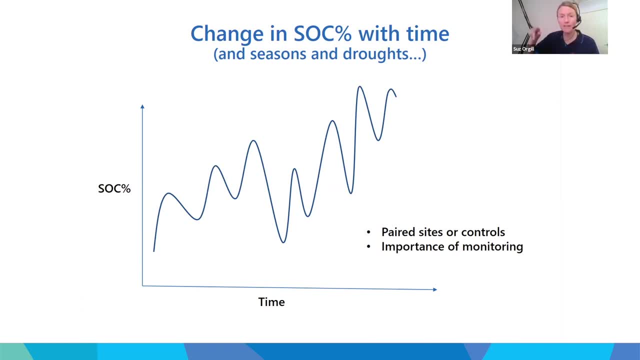 influenced by rainfall and temperature. So we know that this happens. So when we look at the trend over time, if, for our example here, if we changed practice and we were monitoring trends through time, we could see that we've got a gradual increase in soil organic carbon. But if we came in 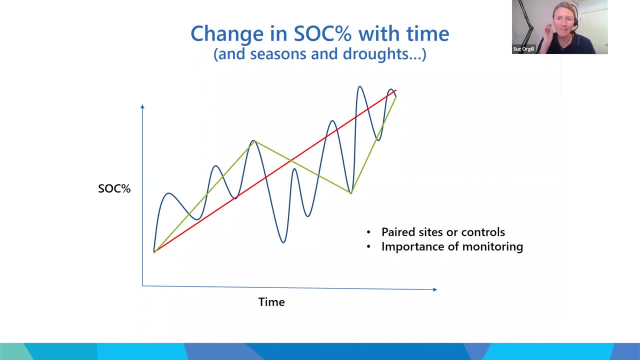 and sampled at different points within that. so if we're only going to sample three times, for example, we could see, maybe think that there's a decline, or perhaps it's not increasing as much as we thought it was going to increase. So it's really important to monitor over time Where you don't 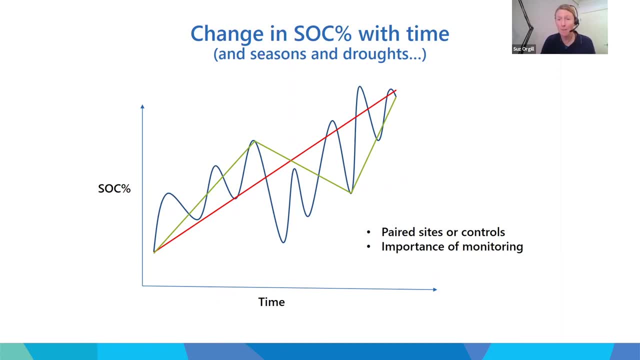 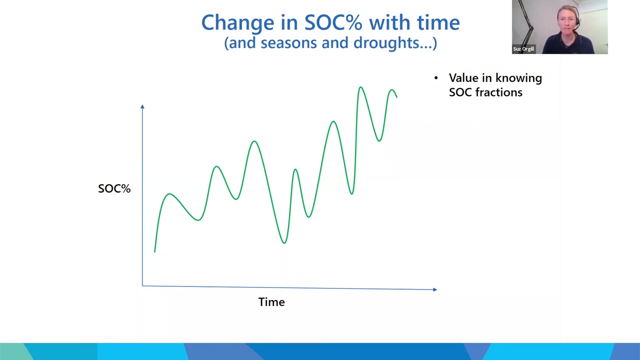 have that opportunity because we don't all have long-term trials. paired sites and controls is a really valuable way in picking up some of that noise as well. Now, another way of picking up some of that noise is looking at our soil: organic carbon fractions. So before, remember, I said: you've got. 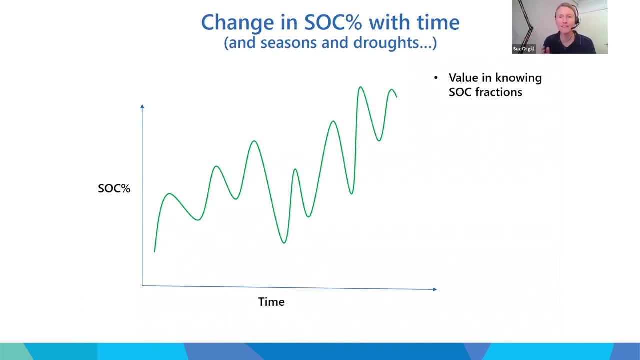 your humus and your particulate organic carbon, and somebody's already hit the nail on the head and said it's the particulate or the label carbon that bounces around the most. So if we think about our char, as I said, this is accumulated. I'm not talking about biochar here. we can talk about that. 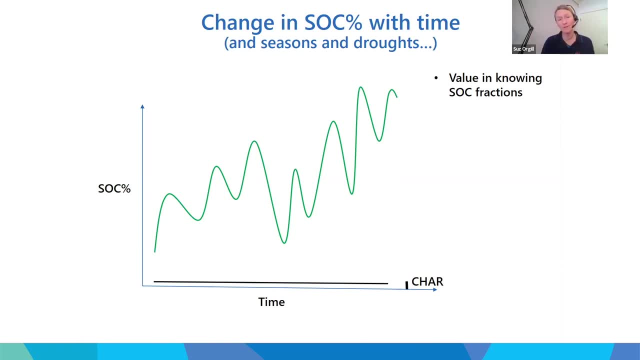 later. perhaps this is looking at char. that's naturally within our soil and doesn't really change. It might be eroded and physically removed from the site but in terms of being stable it's quite inert and stable in our soil. If we've had a management practice change, which I'm suggesting in this conceptual example, 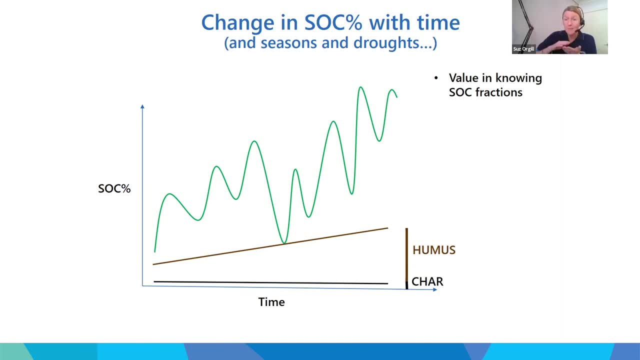 you might get an increase in humus over time. So we can see it builds really, really slowly but it can increase with time and with microbial activity in particular and nutrient supply. Now what we're looking at for this third fraction- that bouncing around most of that variability- 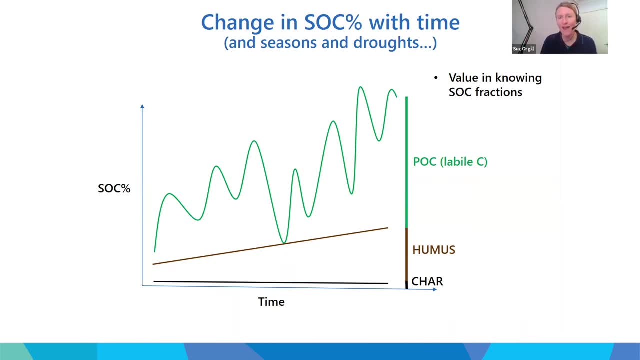 happens in that particulate organic carbon fraction, And this is where, with trading, they've gone back and forth about which fraction should we actually be monitoring For production. the cash is in the particulate organic carbon, because that's where the energy and the nutrient. 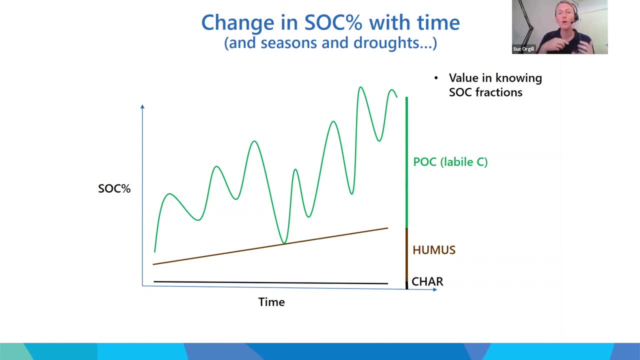 supply comes from. That's where the microbes are really active. Humus is the product of that. So as microbial activity increases, you'll get an increase in humus. but it's very, very slow and it's very, very hard to detect. But there is immense values in monitoring fractions. So if you 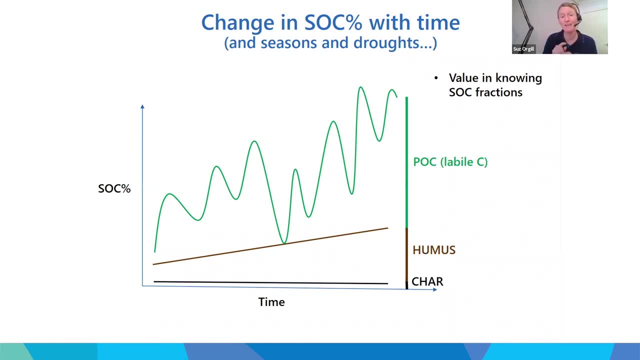 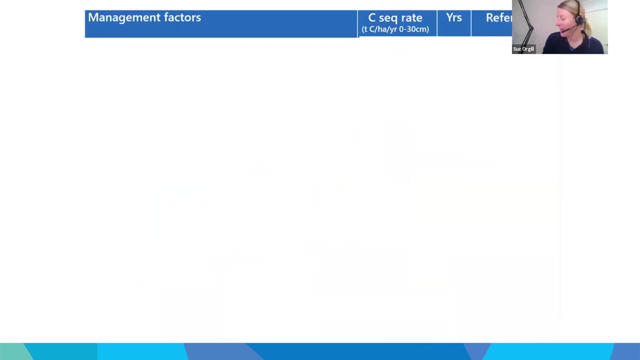 were going to look at your total organic carbon and your particulate organic carbon, you might actually pick up in some of that variability that we get with time. So now let's think about some of the management strategies that do increase soil carbon. When I introduced this yesterday, 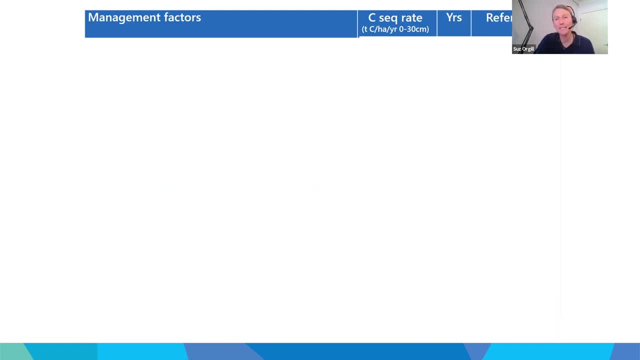 I said how my colleagues who are extension specialists, who some of you may know, say this is a nightmare of a table, but I absolutely love it because it does show you that you can increase soil carbon And the amount of times I've been sitting in presentations and 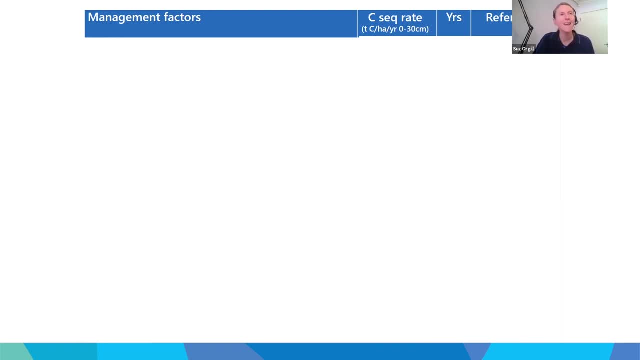 people say it's too hard or it's not possible, or if it's this and that We've got lots of published peer reviewed literature where we do have sequestration rates which have been reported And there's so much that hasn't been reported. but it does depend on seasonal rainfall, on climate and 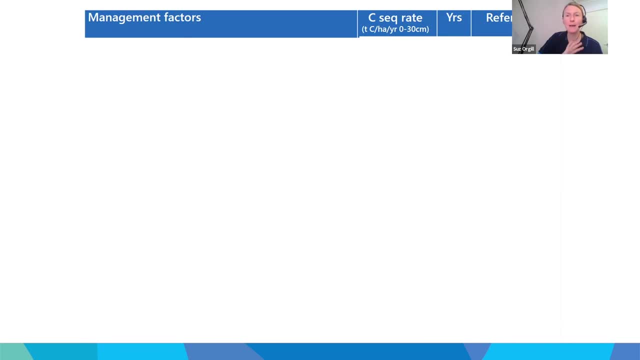 on soil type. Now in this table, before the big reveal, you'll see that I'm going to have a range of management factors. Then we're going to talk about the carbon sequestration rate. So this is looking at the tons of carbon per hectare to 30 centimetres, the years over which the trial was run and the 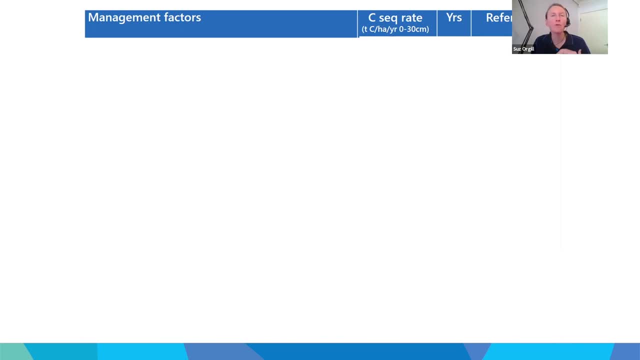 reference which I can provide for people later. Now, the reason it's important to think about the years over which the trial was run is that the carbon sequestration rate generally looks at carbon stocks at the start of the trial, before you change anything. 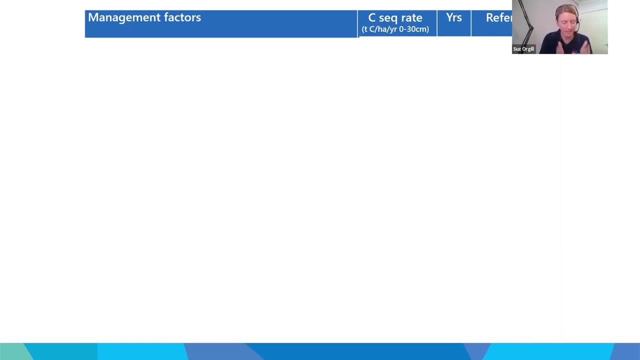 And then the change in carbon stocks over time. But if we just take carbon stocks at the start, this is where we ended. 10 years later, you divide that difference in soil carbon stocks by the amount of years over which that occurred And that's your carbon sequestration rate per hectare. 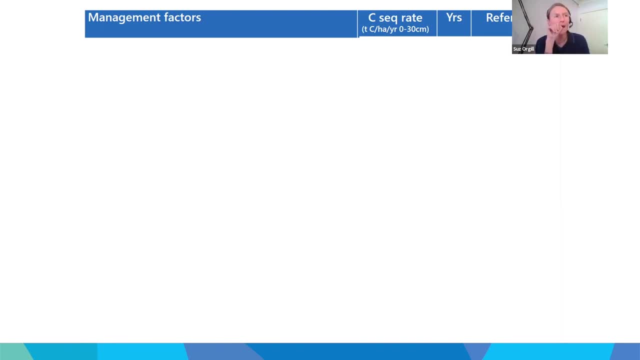 per year, remembering that it would bounce around. Now, most when you change management practice, most of your change in soil carbon sequestration happens in the first five to 10 years and then it plateaus out until you get another disturbance in the system And then you might get another. 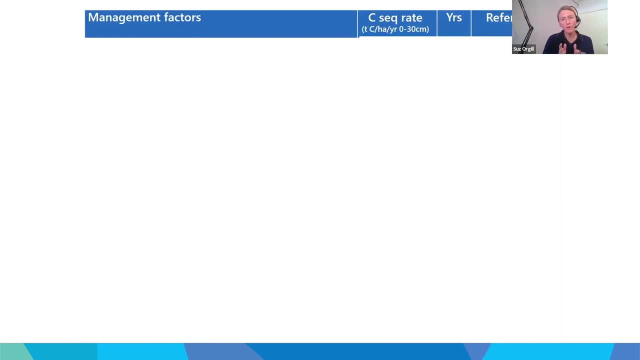 little kick up and another little disturbance and kick up. So if we've got a trial that's only run for five years, and we're talking about two and a half tons of carbon per hectare, you wouldn't necessarily expect that to be maintained for the next five to 10 or 20 years. Okay, So big reveal. 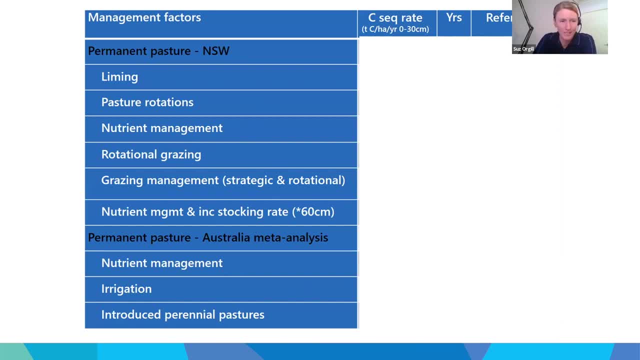 These are the types of practices that we're going to talk about for pastures to begin with. So for perennial pastures, looking at liming, the role of perennial pastures in rotation nutrient management. so making sure that you've got adequate pasture nutrition so that you can grow more biomass to store more carbon. and then 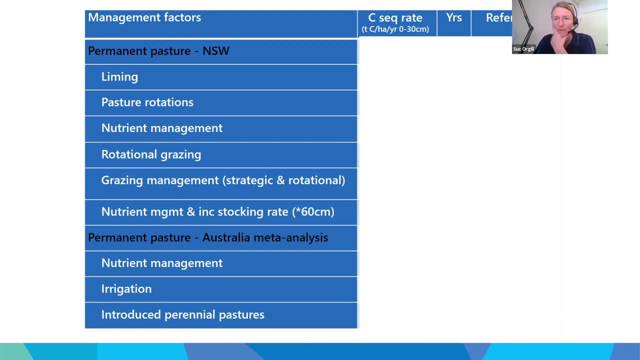 different types of grazing management And there's a whole heap of labels that we could get kind of tied up with talking about this. but in terms of looking at making sure that pastures are grazed so that you've got actively growing pastures for a greater period of the year, And then things like 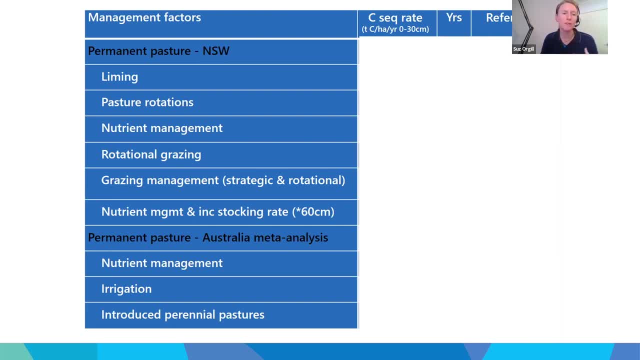 there was a meta-analysis which we'll talk about, some of those rates for things like irrigation and introduced perennial pastures as well. What we can see straight away looking at down this list is there's no spooky science here. It's looking about like a lot of the trials have. 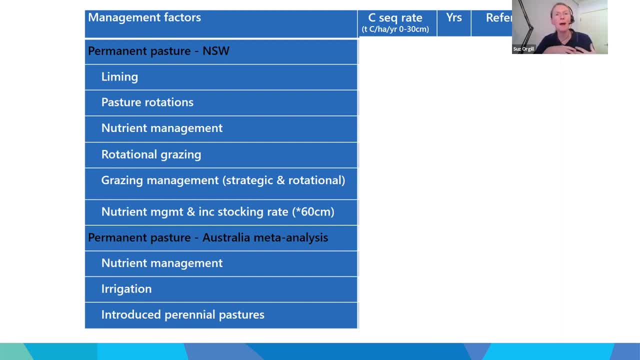 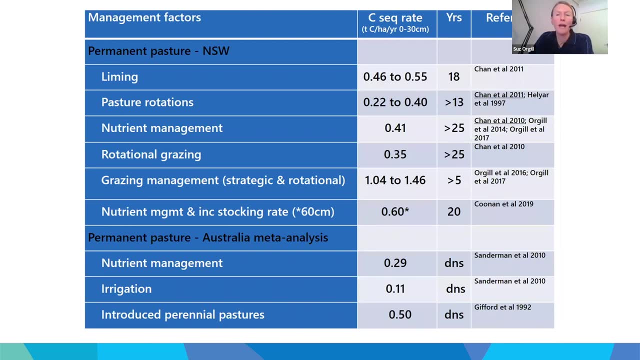 just looked at overcoming soil constraints to production, So making sure that you're maximising biomass supply. So when we look at our rates here, generally they've ranged from point one tonne per hectare per year up to one and a half tonnes per hectare per year. Remember I said the 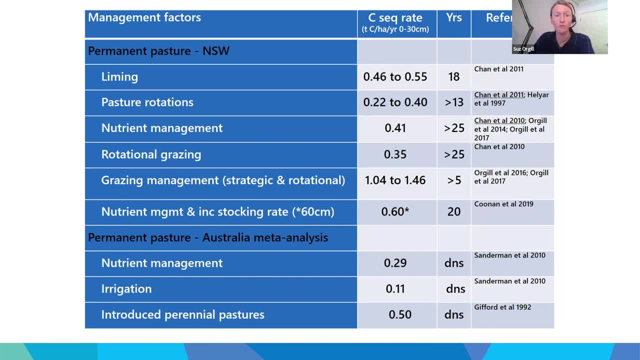 key is to look at the years over which the trial was run. So if we look at the liming trial, which Yin and Mark Conyers ran down around Wagga, that went for 18 years and they managed to maintain over that trial about half a tonne per hectare per year, which is still a significant amount of 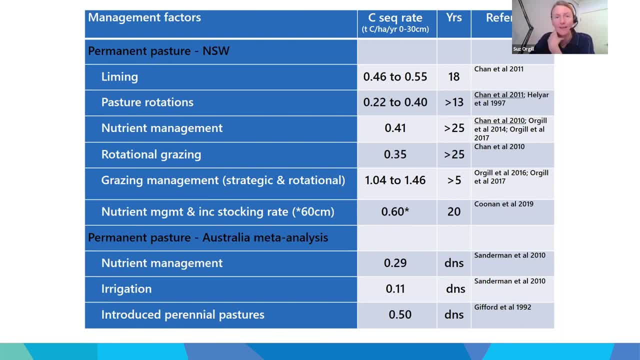 carbon, a significant sequestration rate for an environment like this, Like Wagga. So some of the grazing management that we're looking at there, so that 0.3 tonnes from Yin's work that was in the tablelands environments. For those of you who 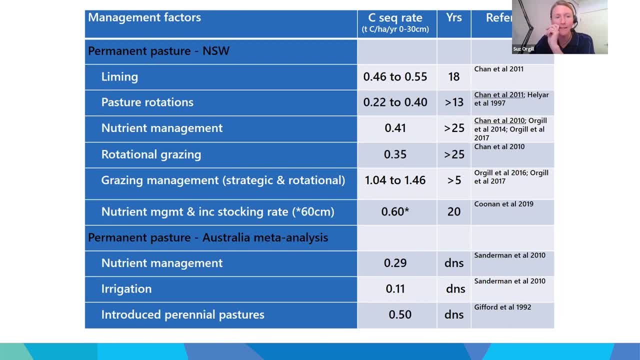 are from the central tablelands and around the Hunter, that would be the case as well. The strategic and rotational grazing management: some of my work that's been done down on the Monaro with five-year actually kind of penned trials with livestock through to some of the 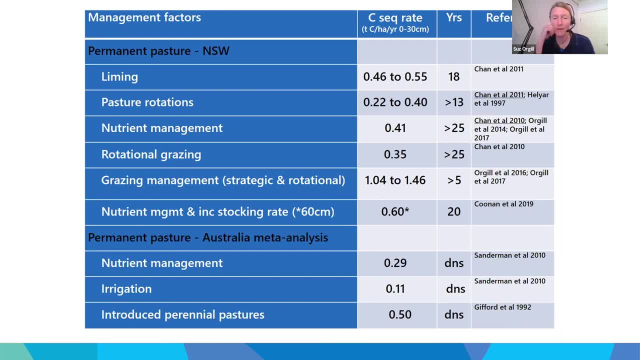 rangelands work, Where we've looked at monitoring sites now for over 10 years and we've managed to identify almost one and a half tonnes of carbon per hectare per year in the low rainfall zone. So it is possible right Now. would this be possible across the whole landscape? No, 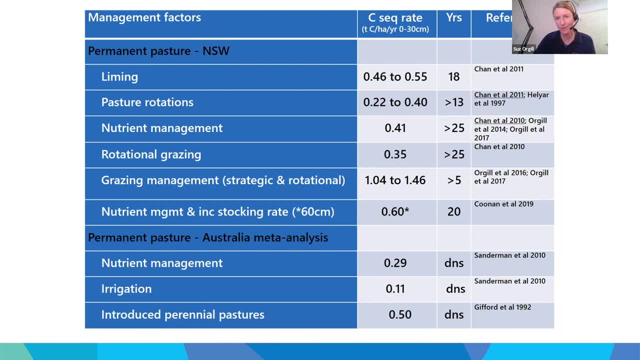 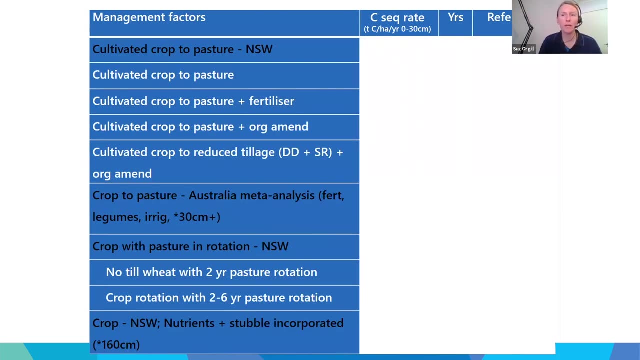 because what you need to do is identify responsive zones, And we'll talk about some of those other limitations in a minute. but thinking about the right practice at the right time in the right place is key here And now. if we just move on to looking at some cropping systems- and I haven't a lot of my 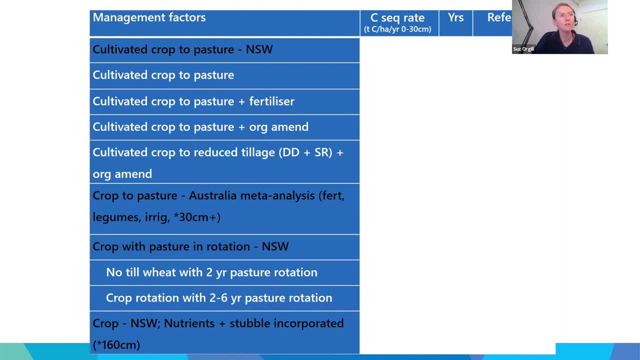 examples revolve around the role of pastures in mixed farming systems or pastures in rotation, because that's the easiest way to build up soil organic carbon and to maintain that biological activity, because it gives diversity in carbon input, it enhances soil structure and aeration. 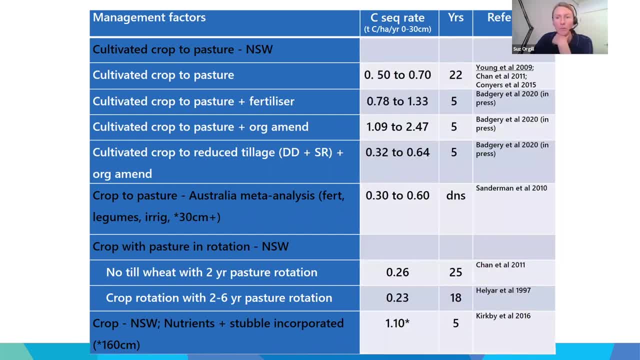 But we're looking at from here. there's been some recent work which we've just published and should be out in the next week or so, where we've looked at converting degraded cropping paddocks. So the key there is degraded, so we're starting from a low level already of soil organic carbon to permanent pasture with adequate 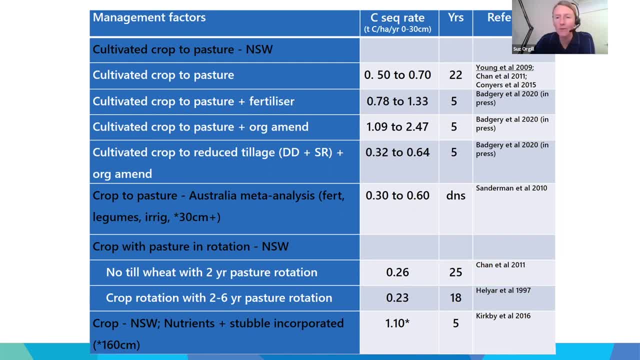 nutrition, And that nutrition doesn't matter if it comes from a bag, from fertiliser or an organic amendment, So just making sure that the pastures and microbes have the nutrients that they need to grow. When we've looked at some of our trials- which I thought last night I probably should have- 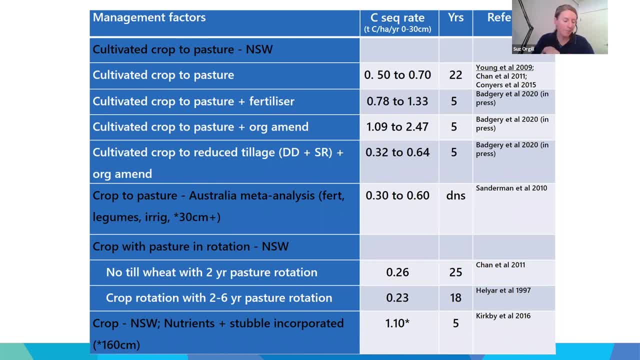 included it for today as well, where we've looked at stubble retention and just moving to direct drill. So, looking at minimum till systems, what we've often seen in our replicated trials is that you reduce the loss of carbon but you don't rapidly increase soil carbon sequestration. 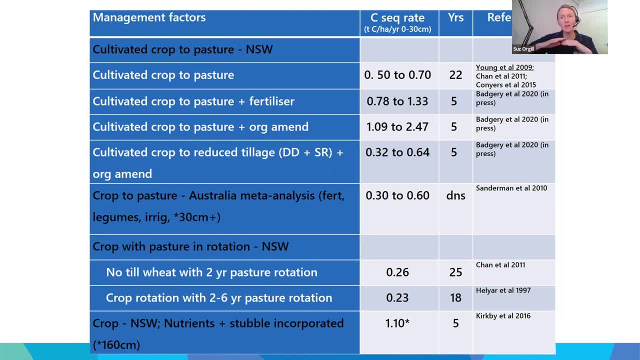 you need something else in the system. So you're going right, we're not going to decline carbon anymore, but what are you going to do? And then you need to think about the role of organic amendments or nutrient management or a biological product, for example, just to kickstart that system. 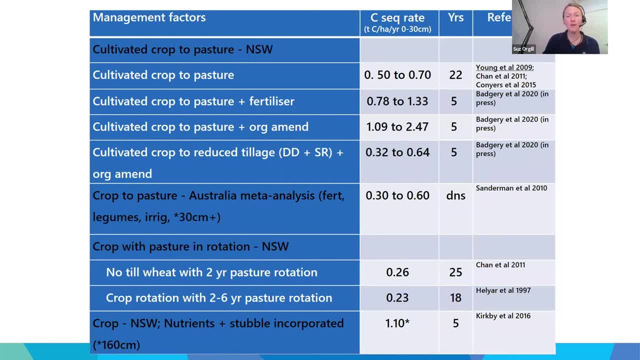 again. So here again, though, a lot of this is looking at that conversion of cropping paddocks to pasture, but also where we've looked at managing the pasture rotation in cropping systems. Again, this is a lot of work in southern New South Wales, where we're looking at about a 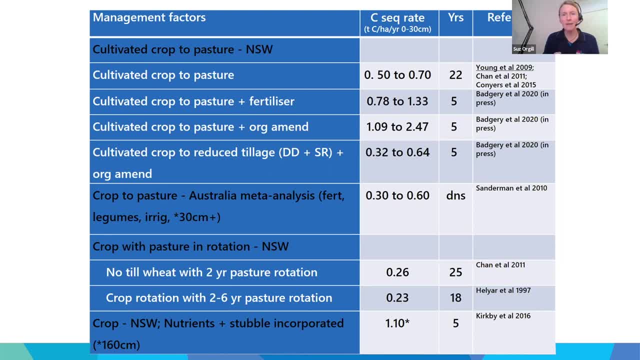 quarter of a tonne per hectare per year. So we're looking at that conversion of cropping paddocks to pasture, but also where we're looking at managing the pasture rotation in cropping systems. Now, some of these might only be two-year pasture phases and up to six-year pasture phases in those. 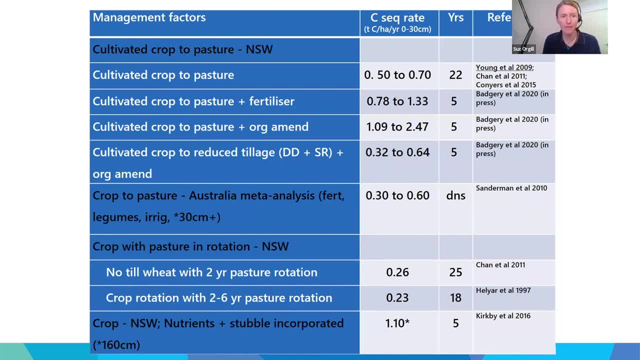 trials Clive Kirkby's work, which is the bottom example there, where he's reported or published over one tonne per hectare per year in cropping systems where you're incorporating stubble with nutrients that occurred over 1.6 metres. So that was. 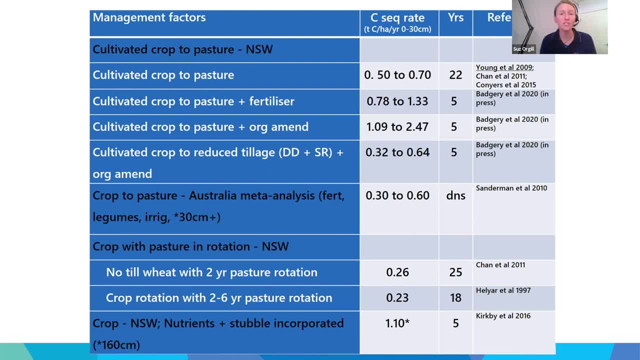 a greater depth of which that change is occurring. and again that was a short-term reporting period so that might plateau off. but again that just shows about the importance of nutrient provision for microbes to decompose organic matter and stubble. But then there's lots of examples where, despite best management, soil organic carbon doesn't. 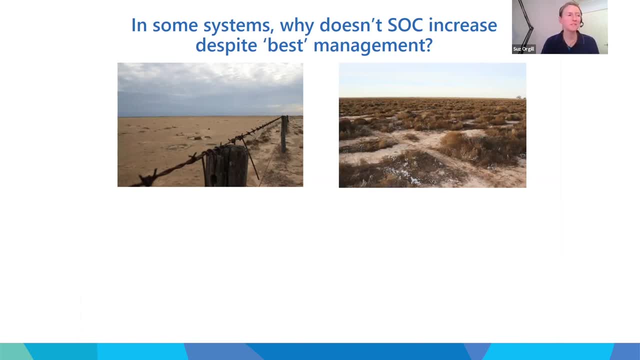 increase. And these pictures here on the screen break my heart because it was one of my favourite. it was one of my first studies where I ever looked at the role of cell grazing in the western division. the left hand picture was a continuously grazed pasture. it's not much pasture left yet. 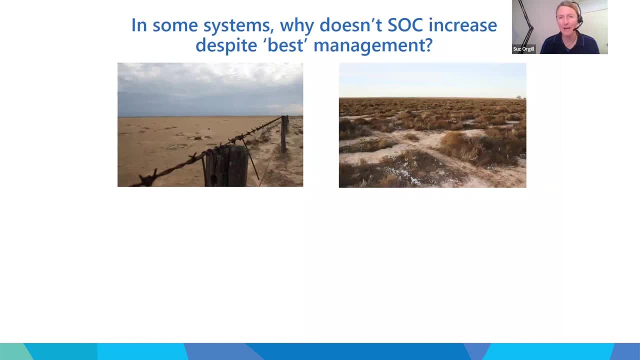 and the right hand side was a cell grazed pasture which had been so grazed. we looked at it for over eight years and if you look at that just by your eyeballing, you'd say, yeah, there's probably going to be more carbon under the place where plants are growing compared to the place where plants. 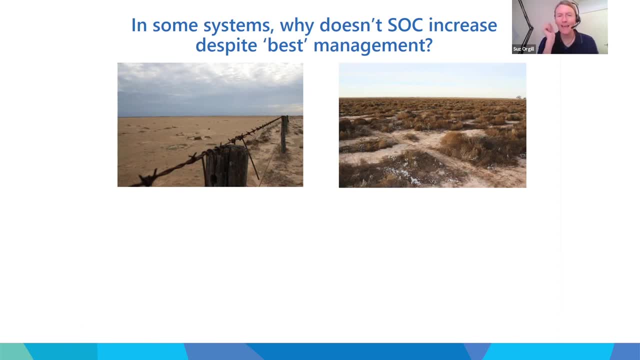 aren't, but there was no significant difference in soil organic carbon contents in that comparison. but if you have a look at it, there's a whole heap of other benefits that are occurring there in terms of ground cover, in terms of feed availability, perenniality in that system and microbial activity. 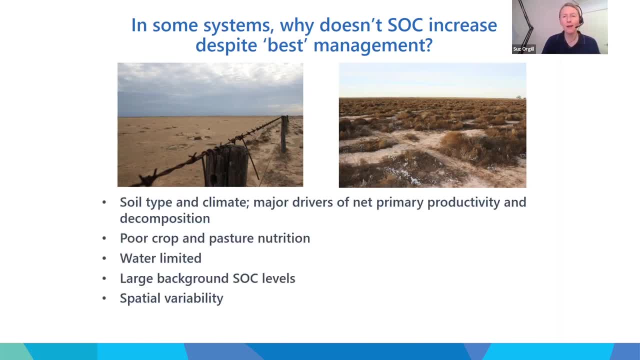 so what are some of the reasons? well, as I've already said, it's really important that you're comparing apples with apples, and soil type and climate can have a major influence on carbon sequestration rates through their impact on productivity and primary productivity and decomposition. poor crop and pasture nutrition is often a cause for little difference in carbon sequestration. 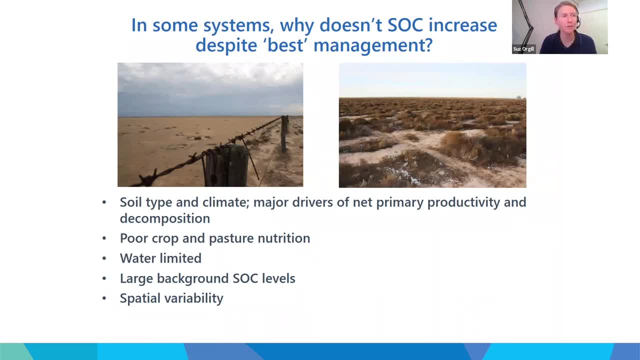 rates. and that's in particular where I've looked at try and some of my own survey work, looking at the role of grazing management and increasing soil organic carbon concentration, and I walked down the silly path myself of going right. well, if we've got rotationally grazed pastures, 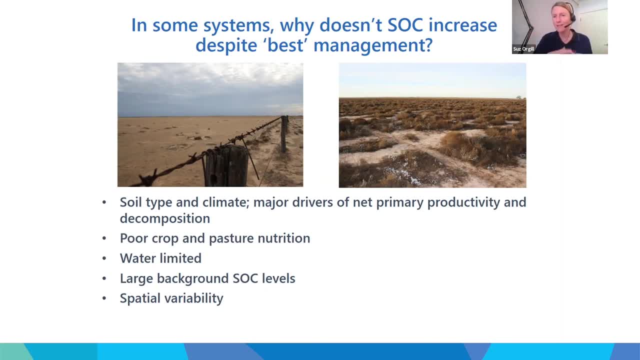 and continuously grazed pastures. of course, pastures which have actively growing plants for a greater period of time can have more carbon, but you need to make sure those plants also have nutrients, and it can be nutrients which can limit carbon sequestration as well. we've already spoken about the kind of bouncing around. 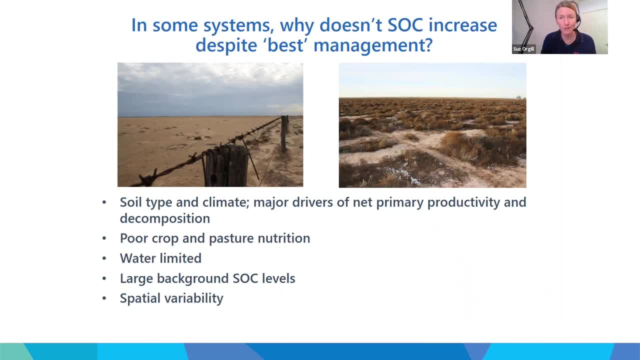 that can happen with, with dry seasons or prolonged periods of dry, with droughts, there's a huge amount of spatial variability, which makes soil science exciting but also makes looking at things like this highly complicated, and it's a really important thing to do and I think it's a really important. 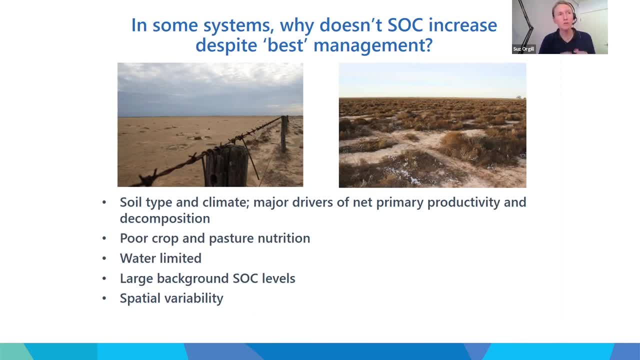 thing to do in the soil science, of course, but it also is a really important thing because it's really very complicated. so you need to make sure that your sampling strategy and design is going to be able to cope with variability in soil properties and soil carbon as well. and then sometimes it 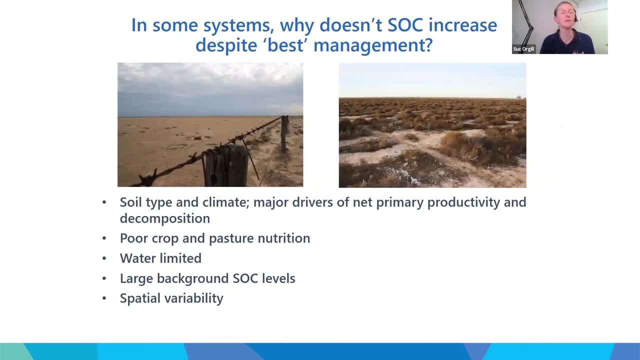 might be that you've already got a really large background level of soil organic carbon. so it's really challenging to demonstrate or statistically prove these incremental changes, and the example that I like to use with this is: imagine if I've got two big soil changes, and it's hard, they may take a while. 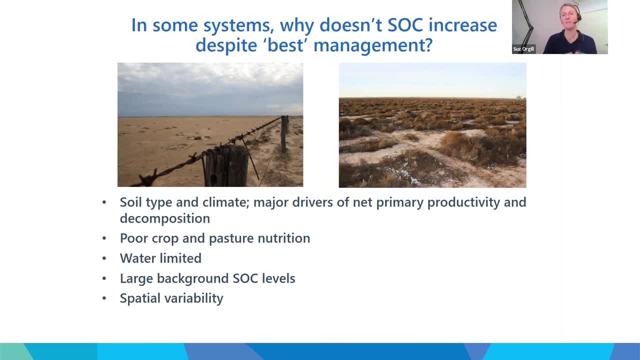 I might just have to put two to three years to get the soil back to normal. so it's a big challenge, but I think that's a very important thing to look at. if you're thinking about Bidwell, I think it's a big buckets exactly the same size in front of me, okay, and at this stage they're both empty, you can see. 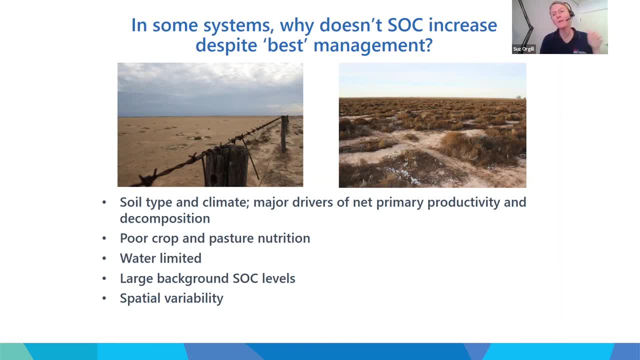 that they're both empty. I take one of those buckets and I fill it up with sand. now, if I get you to look into those two buckets, you go, yep, one's full of sand, one's empty. now if I come along with one cup of sand, okay, now if I poured that one cup of sand into the bucket that's already full of sand. 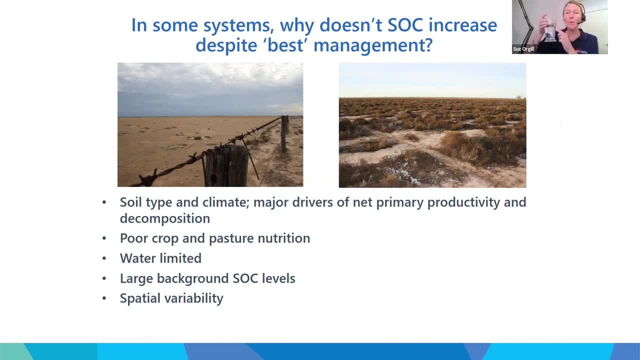 you couldn't tell, could you? no, you wouldn't know. if I poured that cup of sand into the empty bucket, you'd be able to look in and see it. it was the same amount of sand, okay, but you can see it in an empty bucket, but you can't see it in a bucket that's already full. and that's the same. so when 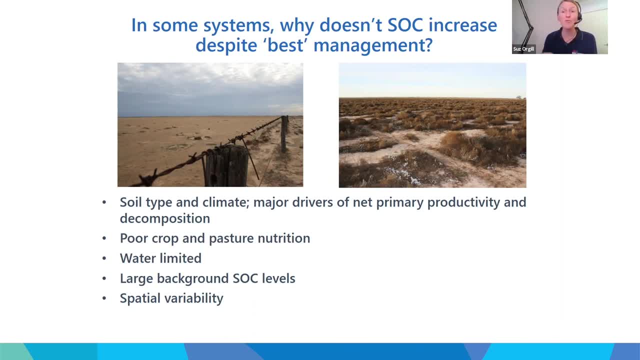 we talk about carbon sequestration rates. it might be the same rate of sequestration, but if you've already got a large background level, it's really. it can be really challenging to detect that, and this is often what we find, where people already have perennial pastures in place with a high nutrition and they're bang on with their. 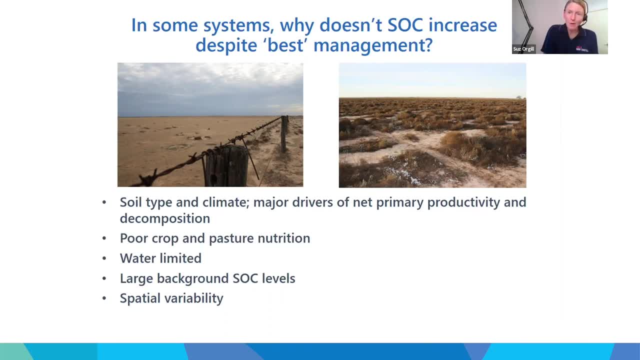 grazing management and we come in and we look at baselining now and looking at increases into the future and it's really hard to detect an increase in a short amount of time. and then sometimes- and this breaks my heart to say- maybe soil organic carbon just isn't the best metric. 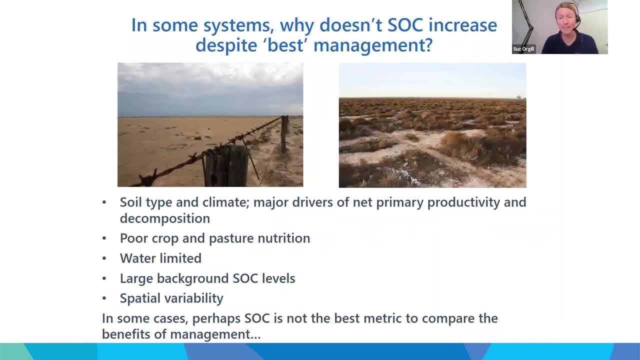 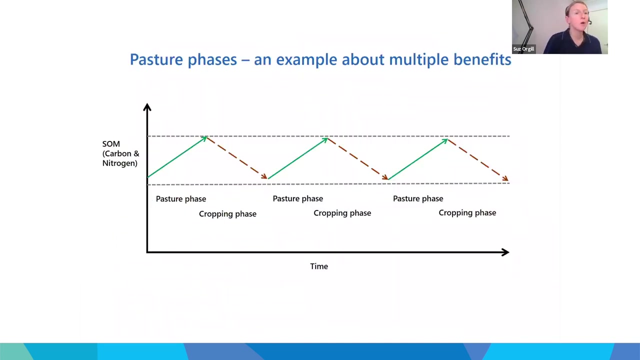 to demonstrate the benefits of management. it's certainly a really important one, but in that heartbreaking impact, a lot of people think that soil organic carbon is not the best metric to demonstrate the importance of rotational grazing, providing ground cover. and so if we just very briefly talk about the role of 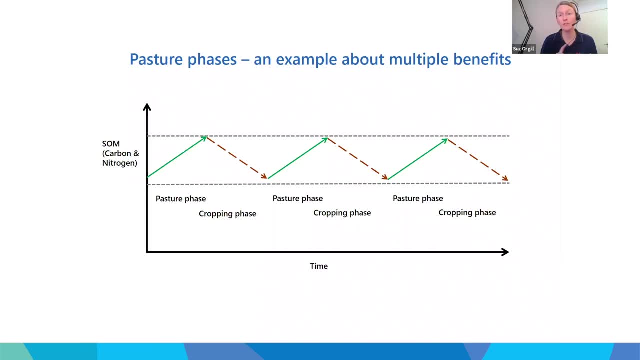 pastures. as i've said, in cropping systems the low hanging fruit is nutrition and pasture. phases for increasing soil organic carbon and pastures are not the best metric to demonstrate the importance of soil organic carbon, and so they are not the best measure to demonstrate a role of natural 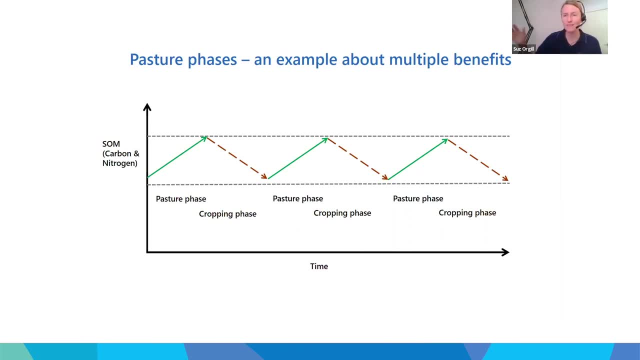 organic carbon, and so we have a really good understanding of the role of organic carbon in soil, organic farming, and so we know that you can benefit. you can benefit from either using organic carbon or using organic nitrogen, but most of the times it can be an issue, because this is a very 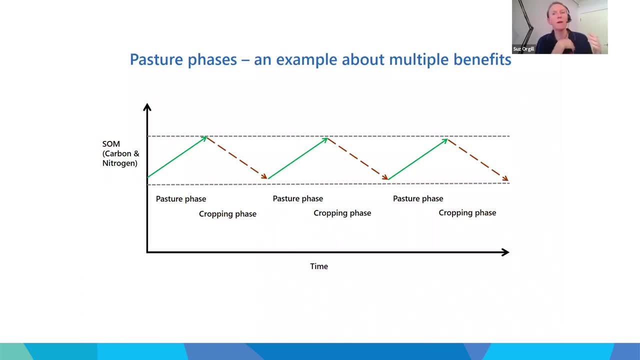 complex diversity and the content of the soil is going to be very different than the content of your soil, and so it's going to be a little bit more difficult to evaluate if you do what you can with soil- organic carbon- than it is going to be the answer you know. again, i mean, apart from the 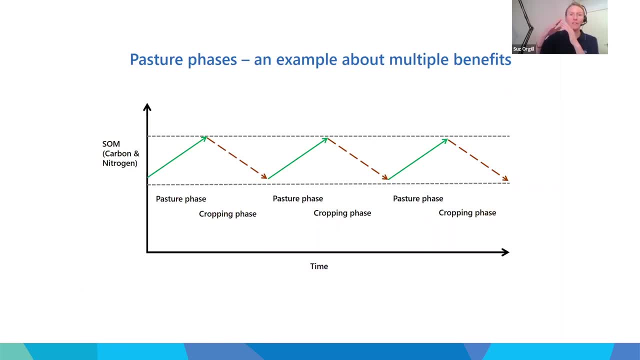 measure of soil organic carbon. it's going to be like you know: you're trying to customize the soil that biologically fixed nitrogen in your cropping phase and you'd get a decline in carbon. Then you'd go back into your pasture phase and you'd increase it again. So you have this kind of 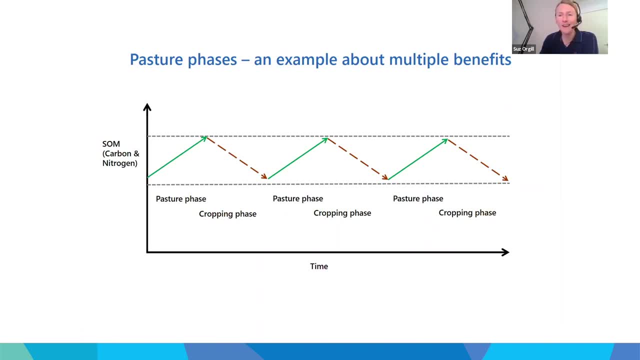 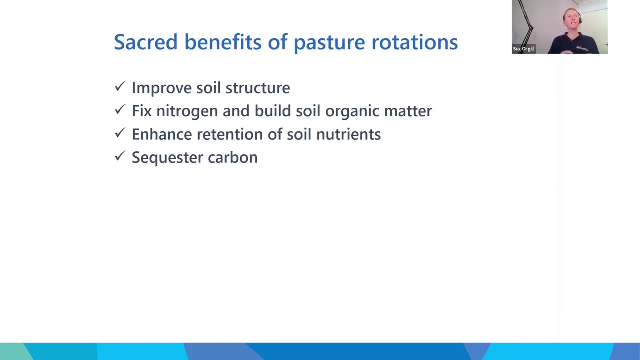 bouncing around. So what can we do here if we were going to try and increase soil carbon as well as get that biological supply of nitrogen? So let's think about it. The benefits of pasture rotations are sacred. They are exceptionally important for improving soil structure, for supporting 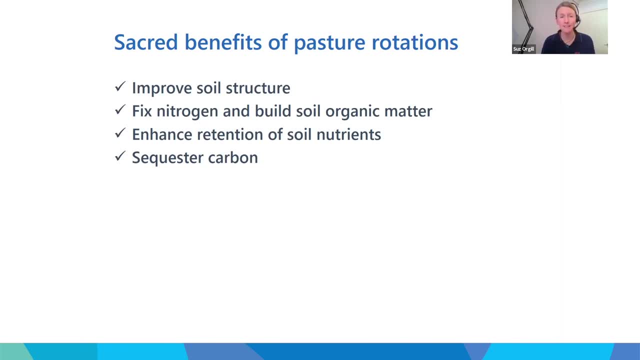 microbial diversity and life within the soil, for fixing nitrogen and for building up soil organic matter. We know that they can also sequester carbon through that accumulation of organic matter. But we also know that good crops need lots of nitrogen and those crops are going to get nitrogen. 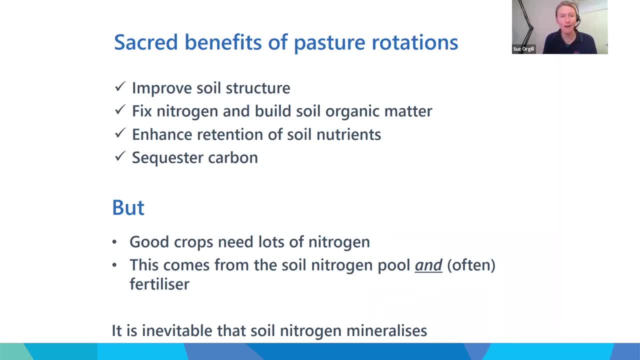 from that organic matter pool as well as any fertiliser that we might add. So it's this inevitable question of how do we get nitrogen from that organic matter pool? So we've got to think about that consequence, that we know that soil nitrogen is going to mineralise from that. 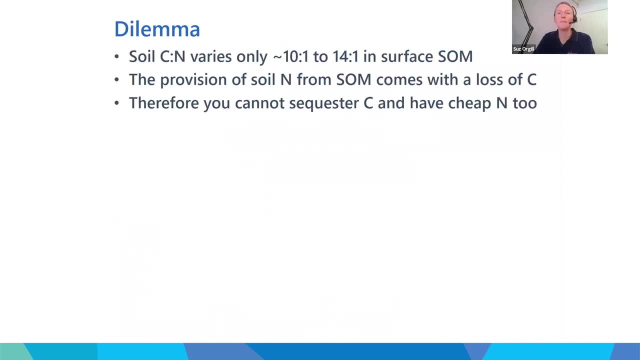 organic matter pool. When we talk about that mineralisation, it comes down to the nutrient relationship in organic matter, and microbes need to decompose organic matter to make nitrogen available and to do that for the following crops, which is agronomically desirable: The by-product. 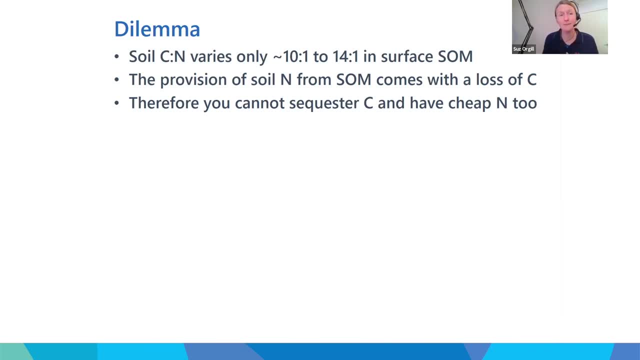 of that is respiration, So we have a carbon loss from the system there. So it's really challenging to have high rates of sequestration with pasture phases and cheap nitrogen. So what am I saying? You need to either alter the length of the pasture phase, the composition of the pasture phase, and or 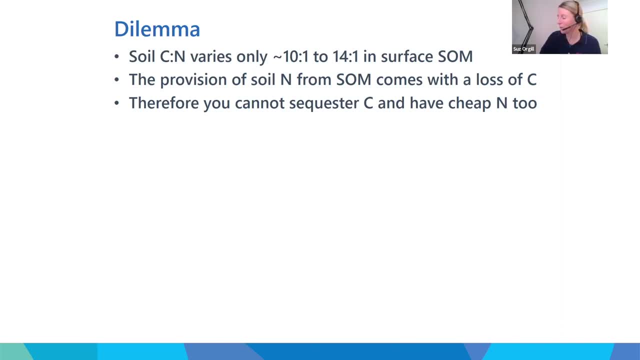 apply nitrogen when you go back into the crop if you want to build soil organic carbon as well. Right, So what are some of our management strategies to build soil organic carbon? Now, in isolation, some of these, some of our strategies, perhaps won't build soil organic carbon. They'll just reduce the loss of. 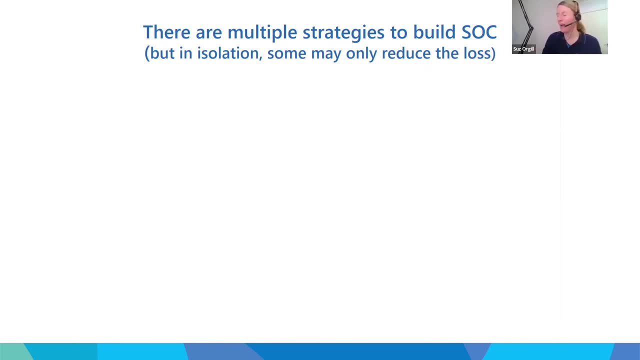 carbon, But certainly some of these are very important in cropping and pasture systems for rapidly increasing soil organic carbon. I've just spoken about the importance of the pasture phase. So changing the crop to pasture sequence can increase soil organic carbon composition. It can also increase productivity in the cropping phase through that role of. 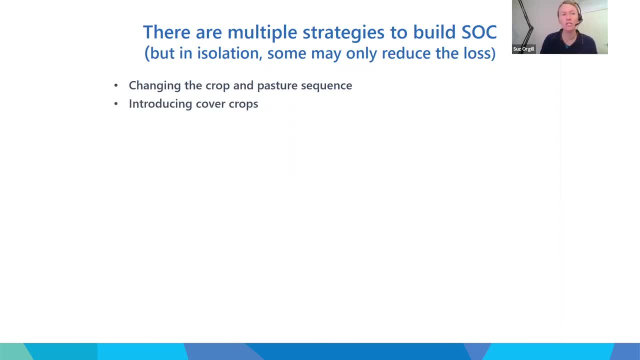 biological production. So that's one of the things that we need to think about. So we need to think about the role of biological health that kind of builds up in soil structure, Introducing cover crops And with a lot of these strategies that I'm talking about in this slide. 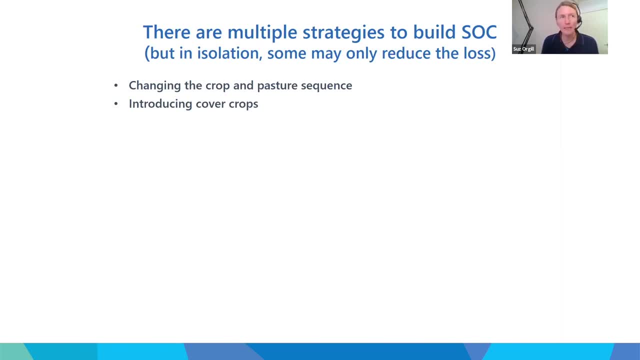 here there might be some short term yield penalties in changing practice, But then there can be long term soil health and productivity benefits as well. So cover crops is going to be have to be decided on a site by site or region by region basis. It doesn't always work because 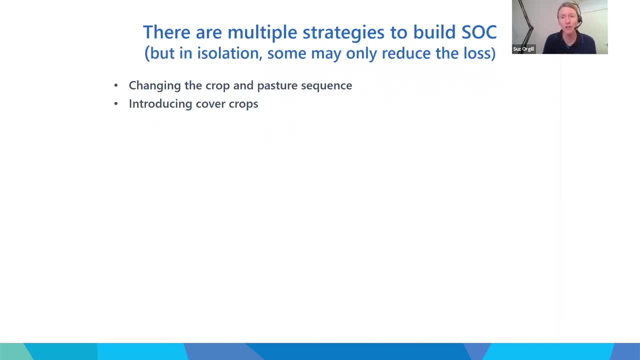 sometimes there's just too much competition for soil moisture when you go into the back into the crop phase. There's a lot of exciting research being done on multi-species pastures in the states and in Australia now, And I think that's going to be a great opportunity for building soil. 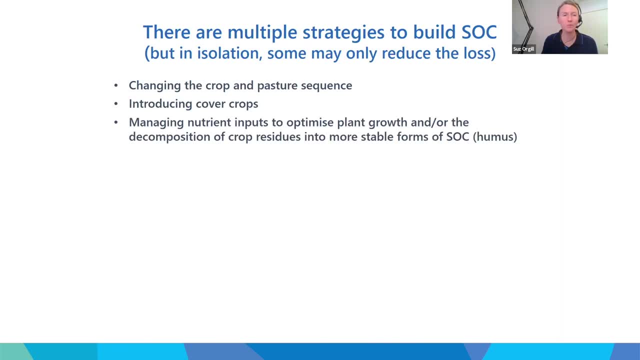 organic carbon and over sowing pastures as well, Managing nutrient inputs to optimise plant growth. growth as well as nutrient decarbonisation, Microbial activity and decomposition. So not only do our plants need nutrients, but our microbes need nutrients as well. As I said, I'm not just talking about nutrients from a bag. Often, I think, 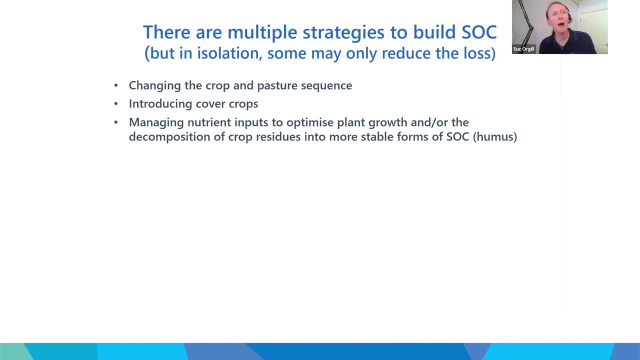 when this work first kind of was a bit of a headline, it was talked about the nutrient value that you need to kind of pay to get your microbes kicking. But a lot of these nutrients can come from organic sources as well, So manures and litters and compost, And they're really important, I guess. 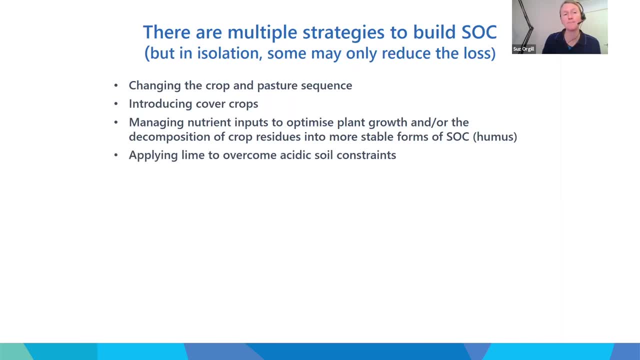 for starting those biologics. Dr Foreverland spoke about the role of the organic matter in advantage of the natural ееquity of your soil and organic matter in the soil. I think one of the most important things we want to see there is the use of organic matter in the soil And we've seen that in the field. So I think that's a huge point and I think that's really important. But I think this work has really helped us. we've shown that the use of organic matter in the soil and building humus Overcoming soil constraints such as acidity and 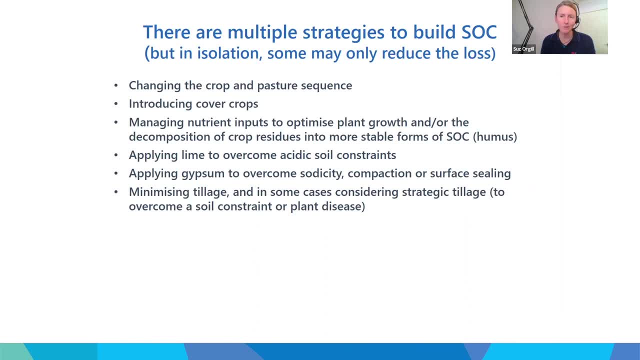 a physical constraint or a biological constraint in terms of like a pathogen or a weed, can actually increase soil carbon, so it doesn't necessarily have to have a net decrease effect Retaining stubble, not only for the organic matter part of it but, really importantly, for the surface soil. 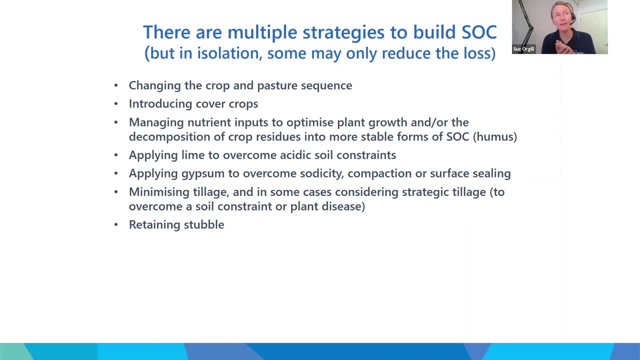 protection from erosion and the buffering that it has with soil temperature, and reducing evaporation loss as well, which is important for our microbial health, Identifying degraded soils or identifying parts which are responsive soils and targeting those. I think, as I've said before, it's not about. 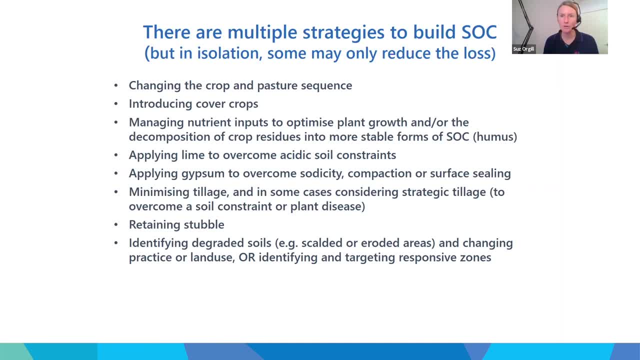 look, thinking about the landscape, and it's just the same sequestration rate, I guess for everywhere. it's about identifying those parts of the farming landscape where you can have maximum increases in soil organic carbon sequestration, or it's just about kind of identifying those parts of the farming landscape where you can have maximum increases in soil organic carbon sequestration, or it's just about kind of. 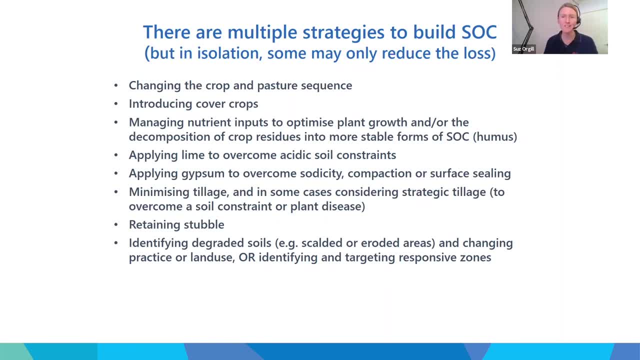 identifying where you want to make those transformational changes and taking it one step at a time and adding carbon rich materials- so things like compost, biosolids and manures- to the soil as amendments, as priming for soil organisms, but also as a carbon source. 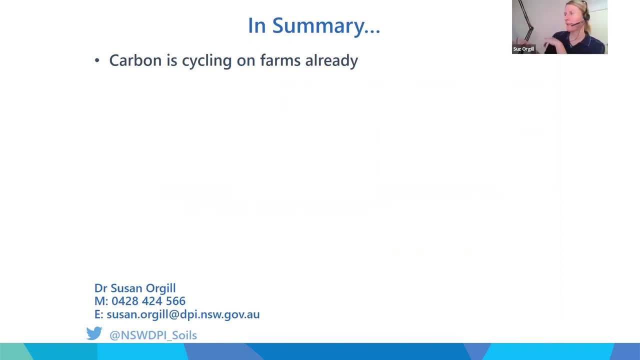 So in summary- and I've got two slides on another one just if we want to talk about soil carbon trading, but just to summarise this part of the talk- so carbon cycling on our farms already and I guess it's available on our other channels as well, and if you want to keep track of those slides, you can. 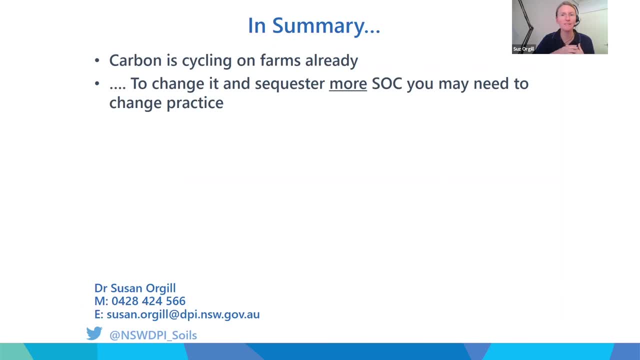 go back to our website and you can get that link and it will be there for you, and the more you can access it, the more you can understand what's going on in terms of how the soil or the soil is going and what you need to do to make sure that you're actually operating in a way that's. 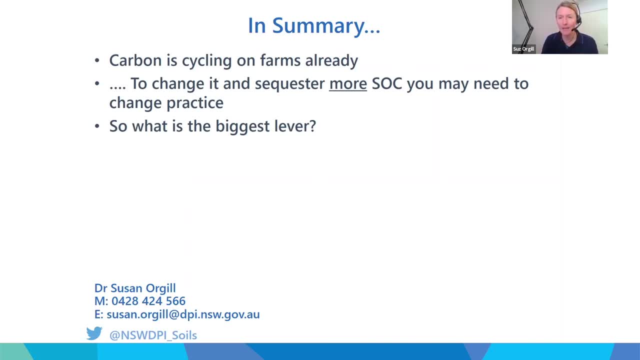 a good place to be, because what you can do is it's the same old way for your plants if you're trying to get nutrients from the soil to the soil, or it's a little bit different, but I would suggest that for soil transportation. So if you're, if you're looking for a third science or a quality soil space or something like that, 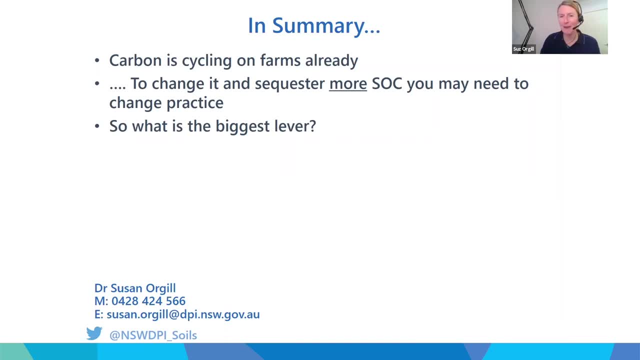 be another constraint might be a constraint in, I guess, decision making sometimes as well. remember, really importantly, that there's soil and climate factors that limit carbon sequestration potential. so when we're thinking about comparing sites between regions, we've got to be really careful and within regions we need to be thinking about the influence of soil type. 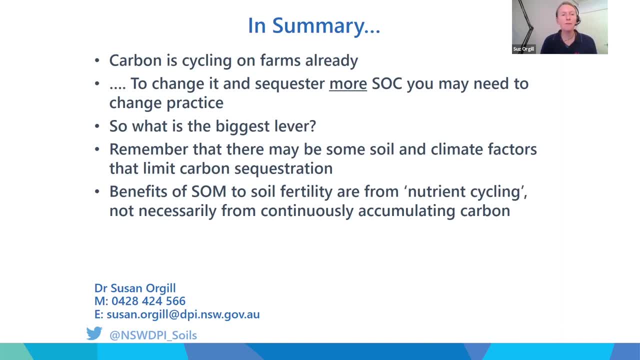 on sequestration rates. the benefits of soil organic matter to soil fertility are from that nutrient cycling. so where I spoke before about the functional carbon, it's not just about continuously accumulating carbon, it's thinking about whether or not your soils are cycling nutrients. so about the microbial activity within the soils, because that's where the value 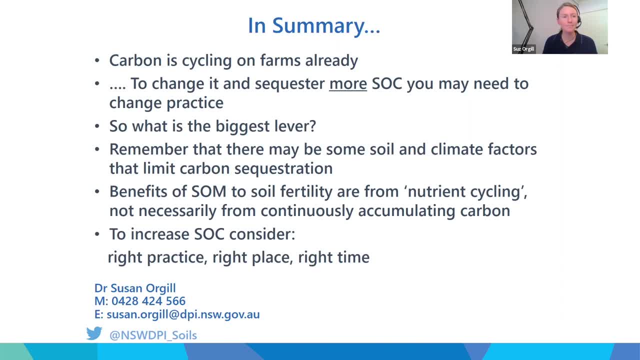 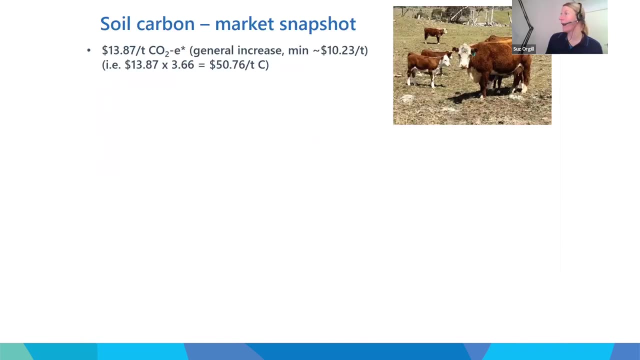 in increasing soil organic matter is and to increase soil organic carbon, you need to consider. as I said, it's about matching the right practice in the right place at the right time. you so I did have. if you'd like, I have two slides on soil carbon trading in Australia. you can trade. 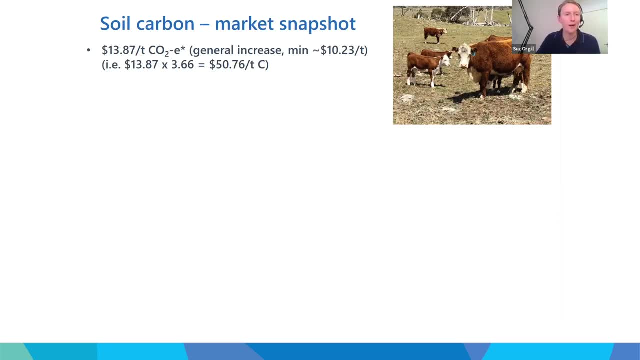 soil carbon. at the last auction, soil carbon sold for, or carbon sold for about $14 a ton of carbon dioxide equivalents. this has been an increase from when the market first came online a few years ago. from $10 a ton in Europe, I think, the price is around $40 a ton. so in Australia the market is quite small and 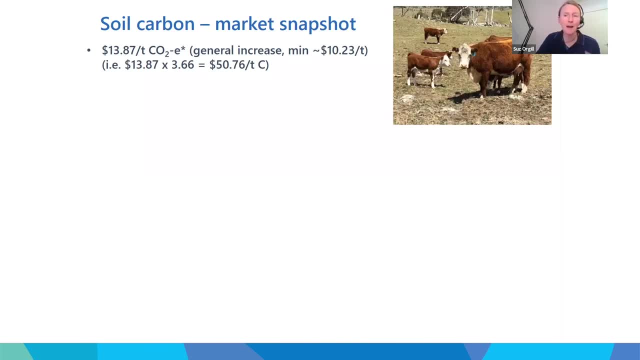 restricted by price at the moment. but remember, this is carbon dioxide equivalents. so when we're talking about, say, $14 a ton or $13.87, we multiply that by 3.66 if we're looking at how much that is per ton of soil carbon. okay, all of us. so I generally say in southern New South Wales with 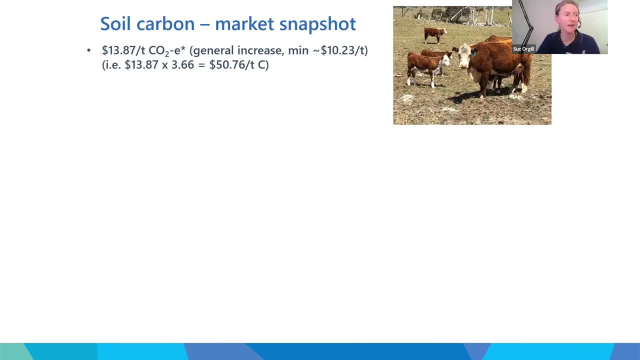 improved land management practice. with change in the soil carbon rate, we're going to be talking about the process of managing soil carbon at a higher rate for every hectare. we're going to do some sub-interest here. now I will be talking about the other issues. I'm going to be addressing this. 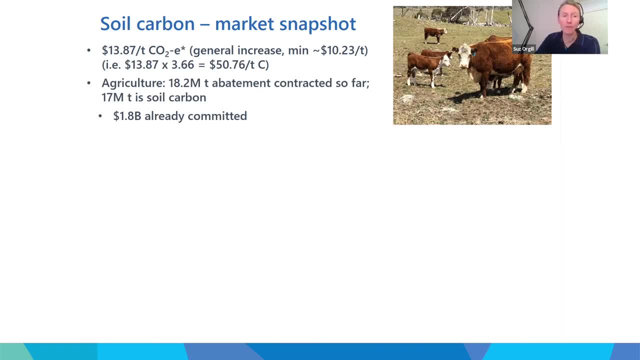 afternoon and I'm going to be talking about the effects of soil carbon in the. have you seen the last poll that we did, where we had a lot of people that were curious about? we're looking at where we've seen some value: that's in soil carbon, and how much does that have to do with the other way? 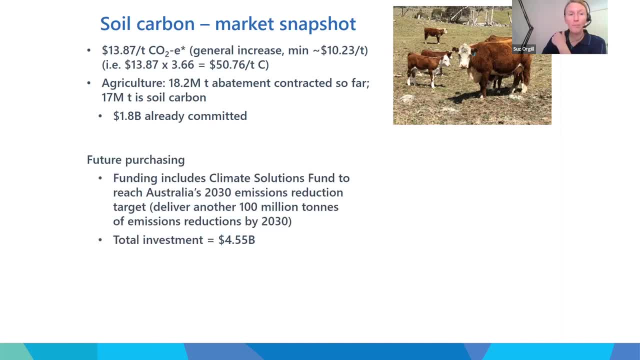 around, like in several areas of the system. in particular they're looking at how much soil carbon may related to your and based on the vision as well. but with the Australian government they've kind of now got the climate solutions fund, so there's additional money that's been put into purchasing carbon from all industries. now the 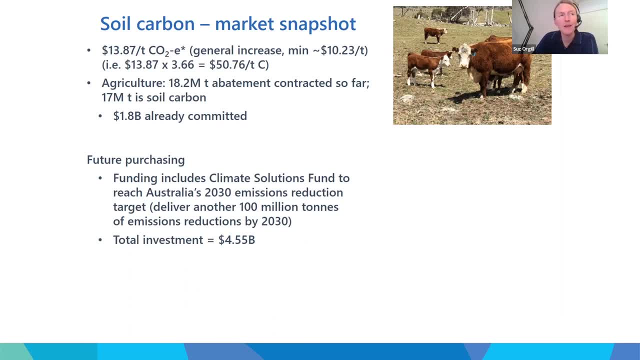 total investment sits at over four and a half billion dollars. it's important to remember, though, your story doesn't really matter when you're selling carbon on this market, and the reason I like to highlight that is because I think consumers, in the end, will start buying the 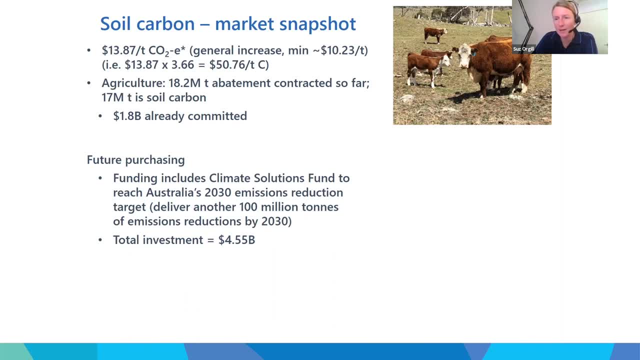 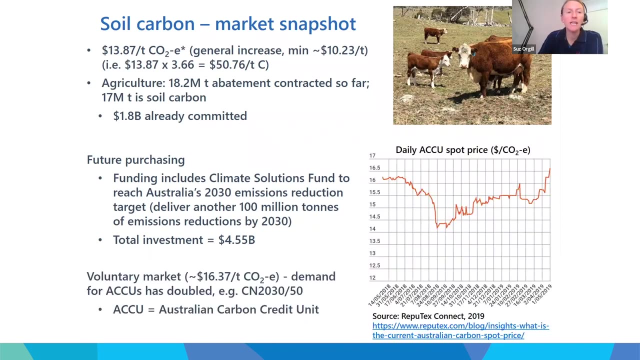 story and the narrative around why increasing soil carbon is important, so all the things that go on with that in terms of improved soil resource condition, and that's where we've got these emerging markets coming online for green kind of green premiums and ecosystem services. to sell carbon, you need to acquire an ACCU, an Australian carbon credit unit. 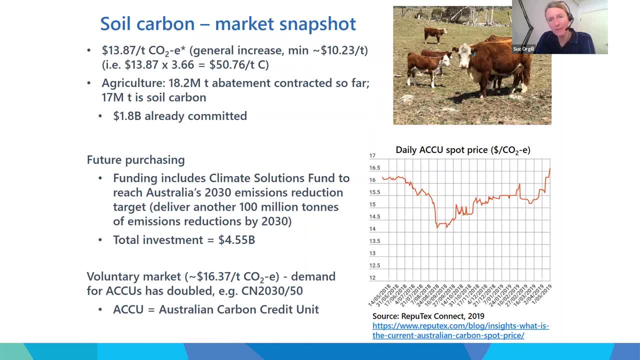 so you can sell these ACCUs to the government and that's that price that I spoke about before, around that 14 a ton. but we've also got a voluntary market in Australia as well, and generally the price on the voluntary market is higher. so why is it higher? because people are buying part of the 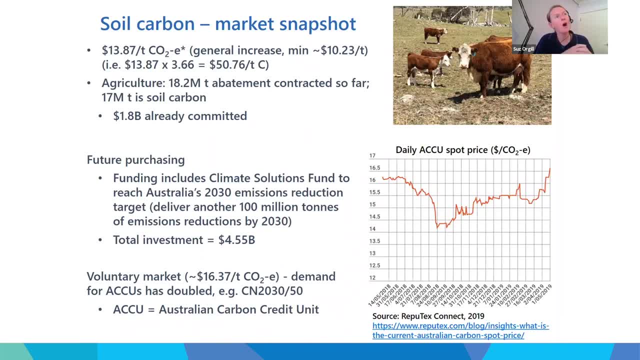 story. so this is where people, where industries, are going. okay, I'm a big airline company and I need to offset my emissions, because I know people are looking now at what we're doing, whether or not that is acceptable. I could buy credits off the government or I could buy it off an aggregator where I can sell some of. 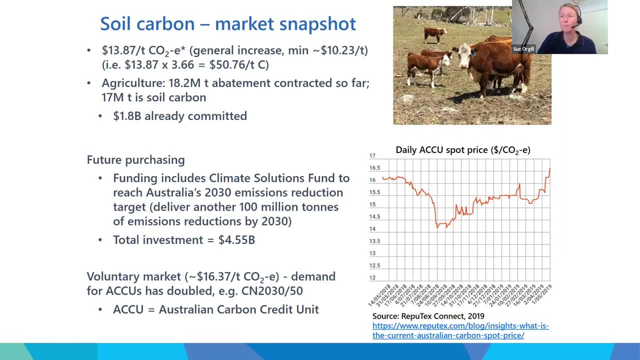 that story and I can tell them that my carbon credits are coming from trees that are planted in this area and soil in this area that's being farmed this way. so the voluntary market is quite attractive for people who don't have to decrease carbon emissions, but it's good industry or business. 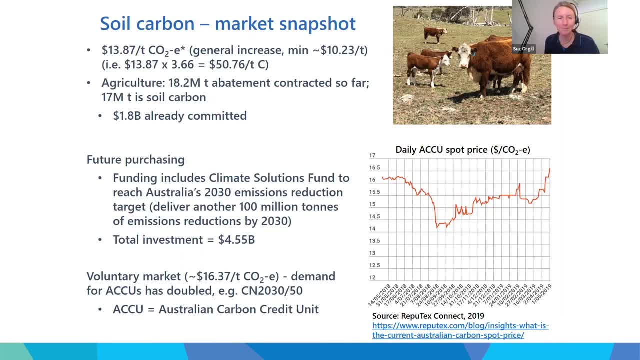 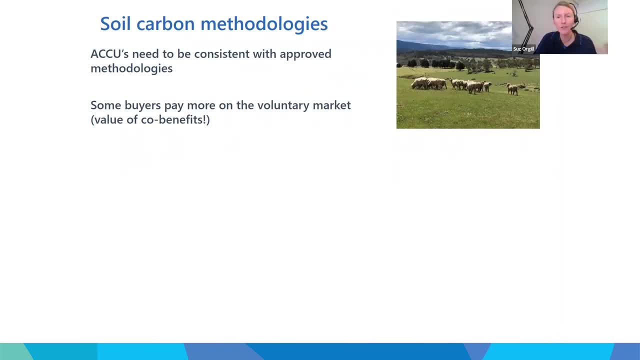 practice to decrease carbon emissions. so the ACCUs need to be. but regardless if it's on the voluntary market or the Australian government market, you've got to get an ACCU so you can't sell it otherwise. and it needs to be consistent with approved methodologies and these methodologies are regulated to the Australian government. so in 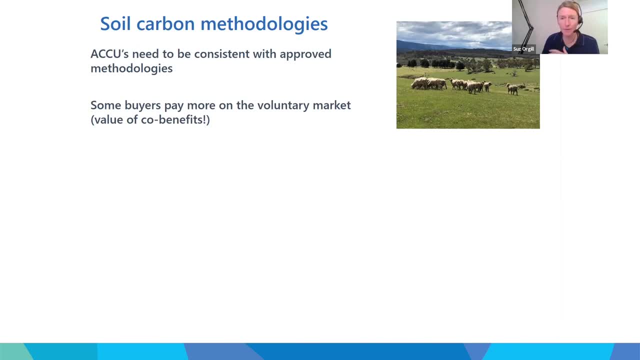 the next couple of months we're going to see massive changes in this space because they're revising all the soil carbon methods and the reason that this is exciting is that they're making it easier for farmers and aggregators to form partnerships in this space to increase soil carbon. 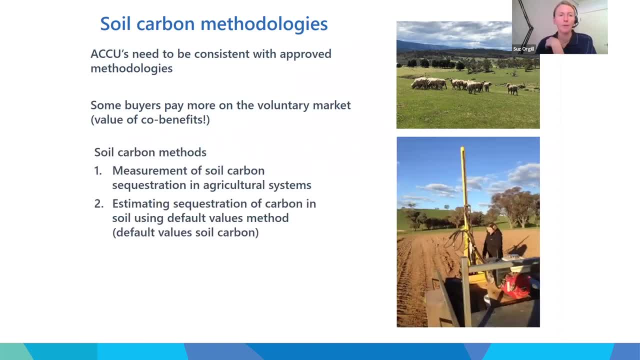 at the moment there's two soil carbon methods. one is a measurement based method, so where you take a baseline measurement- very complicated and quite expensive- and then you demonstrate and then you implement your practice change. then they come back five years later and measure the change in soil carbon and then they do that again at regular intervals and you get paid on the increase in soil. 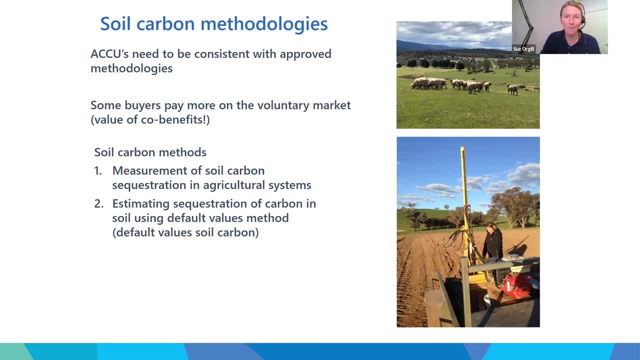 carbon, but when they're selling it to the Australian government it's not going to be the same as when they're selling those credits. they might give you an indication as a producer about how much they think, based on literature and models. now, the models greatly underestimate soil carbon sequestration rates at the moment in a lot of regions. so where we've looked at, 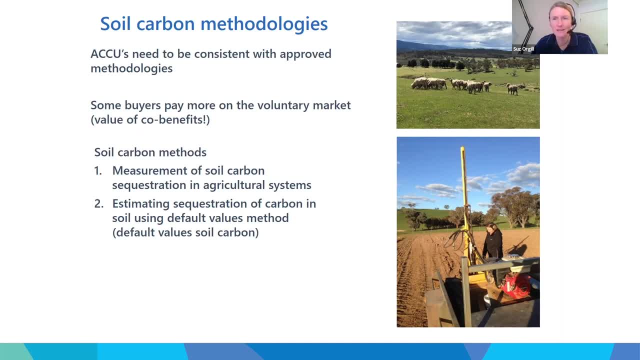 sequestration rates of, say, half a tonne up to one and a half tonnes. in our recent study which is coming out this month, the models are looking at only about, say, 0.2 of a tonne, so they're quite conservative. the other method, so that's the measurement based method. the other method is: 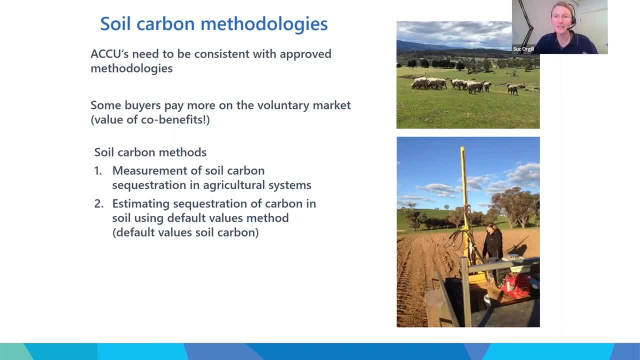 using default values. so this is where they say: okay, you're in this region with this soil type, under this climate, and you're now going to change from a crop to a pasture, or, with your pasture, now you're going to apply nutrients and you're going to graze it so that you're maintaining maximum. 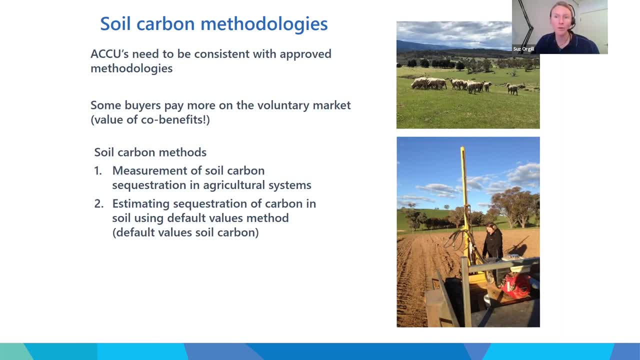 ground cover for most of the year, and then they'll give you a value and you'll kind of sell that. as I said, it's quite conservative though. so there are approved strategies or practices that are on that kind of positive list, and they're all things around overcoming soil constraints, grazing management practice. 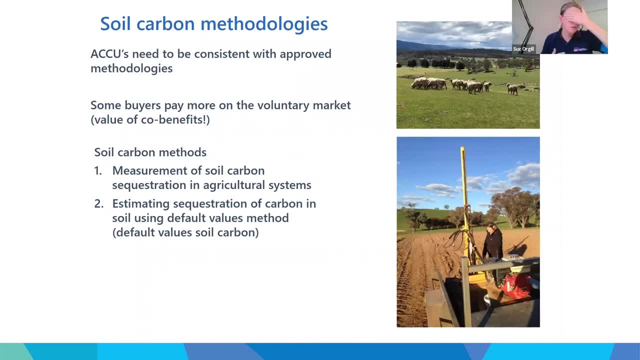 use of compost is on there, biochar is on the positive list, so there's some, and the role of legumes as well is in there as well. um, now, any carbon that you get paid for needs to be additional, so it needs to be an increase if 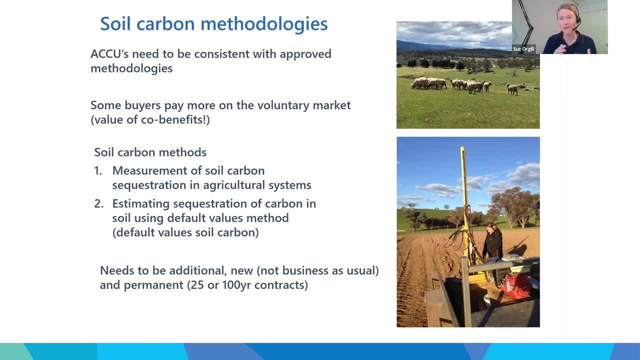 you've got really high carbon levels already. you can't get paid for that. it's only the sequestration that occurs after the contracting begins, and so this automatically kind of rules out a lot of people perhaps who have already implemented best prac. um, it needs to be new. so.